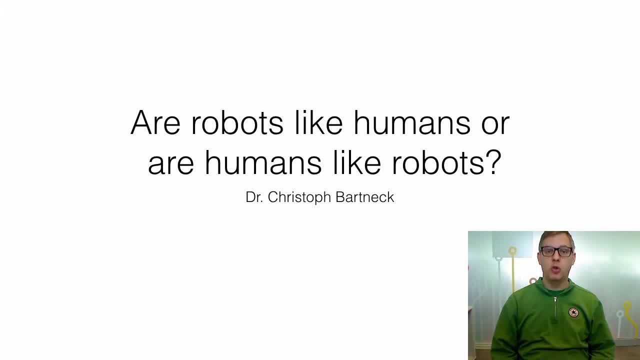 Today, I would like to talk to you about human-robot interaction, which is, in my view, one of the most interesting interactions between users and products. Robots are really behavioural products and their complexity of action and interaction and behaviour they have to show is unparalleled. So one of the topics that I am particularly interested in is anthropomorphism. 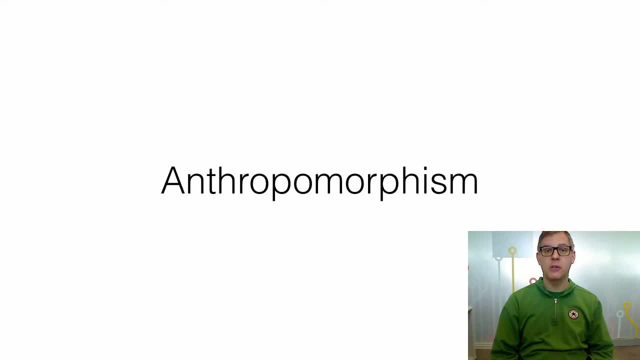 and anthropomorphism is the degree to which humans ascribe human traits to machines, And while we all yell at our computers and call them names, and even have names for our cars. this gets even more interesting when we have machines that become ever so more human-like. 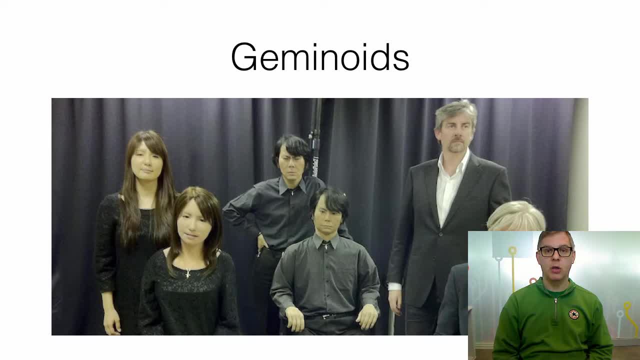 Here you see a series of geminoid robots that were produced by Hiroshi Ishiguro, And the exact goal was to make a copy of actual people. Now these robots are being produced by a company in Japan, and they take very detailed photographs of the skin and the body of all these real 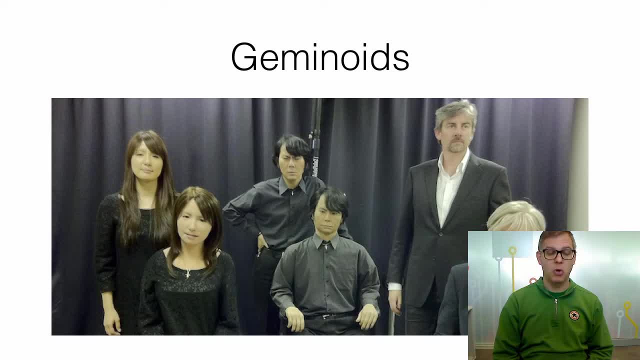 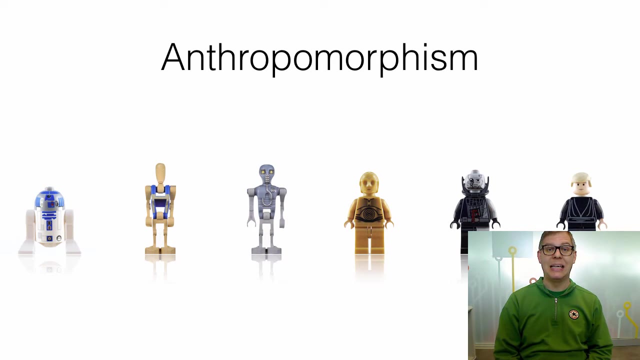 people and then produce animatronic robots that use air pressure for its actuators. And, as you might guess, anthropomorphism is quite an interesting, complex topic, where it is really a gradient. We can ascribe human traits to very machine-like machines and, of course, the more 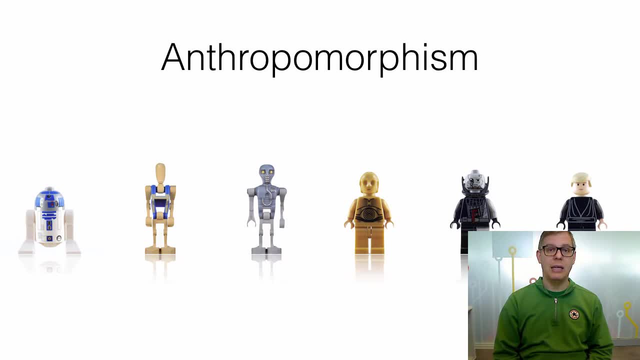 human-like these machines become, the more likely it is that we ascribe human traits to them, And one of the examples I would like to show you is something that happens when I took one of the robots to my home and I just unpacked the popular robot and took it out of. 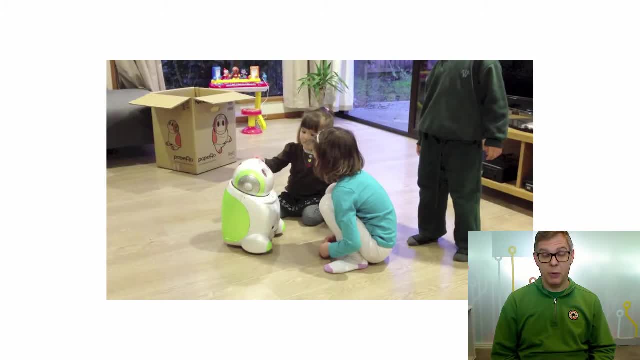 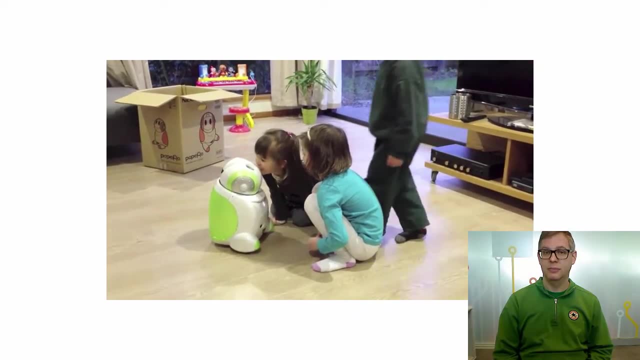 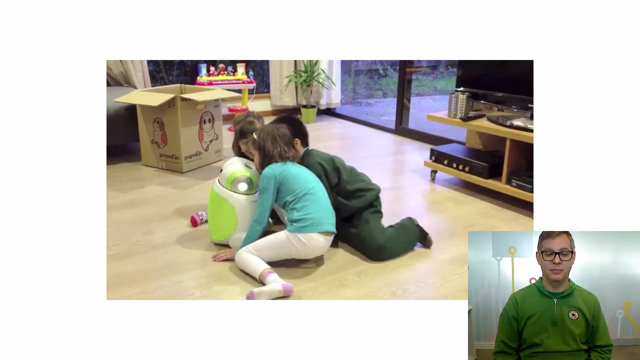 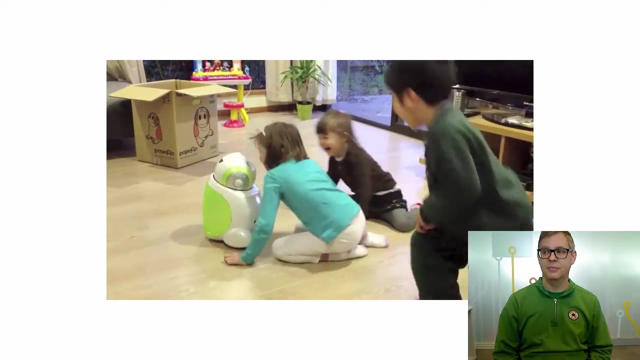 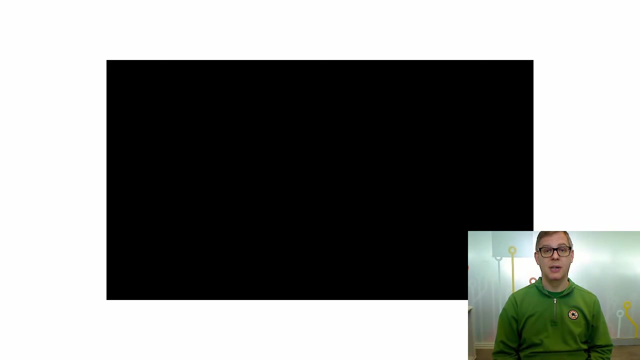 the box and showed it to my kids, And this is what happened. This was completely unscripted, unplanned. The girls just had the idea that this robot was to be kissed And, of course, for a machine or for this particular robot, this was completely meaningless. 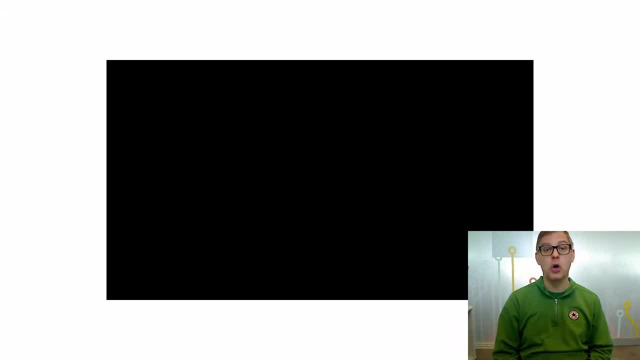 It can't even sense that it is being kissed or it doesn't even know what the meaning of a kiss is. But the children thought that this is the right thing to do, And I think it's a very positive example of what happens when humans interact with robots. And again, this was the first time. 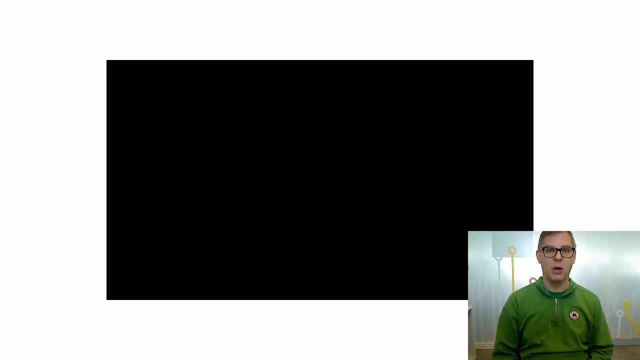 They've never seen this robot before, They've never interacted with it before, And this is the idea that they had about what to do with it. My speculation is that the robot did have LEDs for its mouth, and that might have motivated them to kiss it. Well, one of the problems that you have with anthropomorphism. 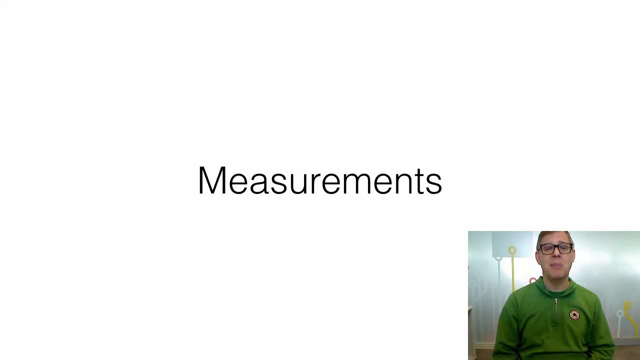 is the ideas or the questions about. well, how can you ever measure that? How can we measure to what degree people treat machines as if they would be humans or at least social actors? And I would like to go through a series of studies that we have done in order to shed some light on these questions. 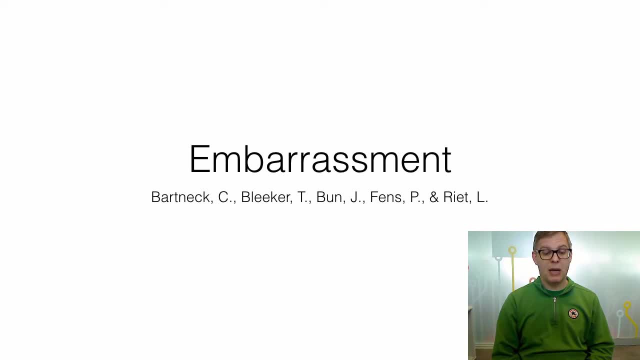 One of the first studies that I would like to talk about deals with embarrassment. Now, when you go at home to bed and you make yourself ready, and maybe you change your clothes and you undress to be able to put on your pyjama and, let's say, you are in front of your washing. 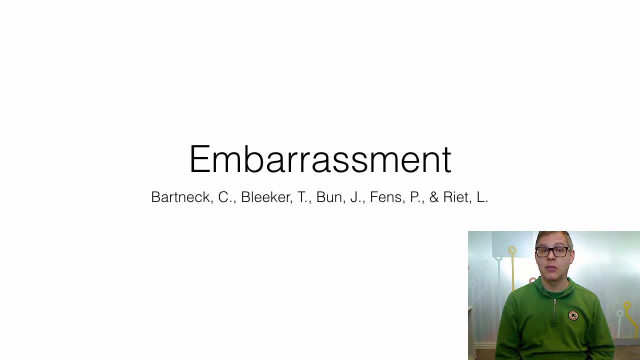 machine. it is very unlikely that you would feel any kind of embarrassment. Now, if I would be in the room and would be observing the robot, I would be very embarrassed. I would be very embarrassed And would be observing you doing this. you would probably be very embarrassed because I'm a human. 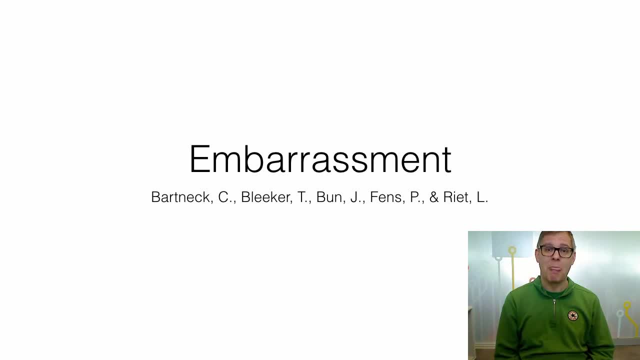 and I'm a stranger and that would be just rather odd. So we had this idea that if people are embarrassed in front of the machines, that would imply that they would consider the machine to be somewhat anthropomorphic. Now we put this into a context of of a medical scenario. 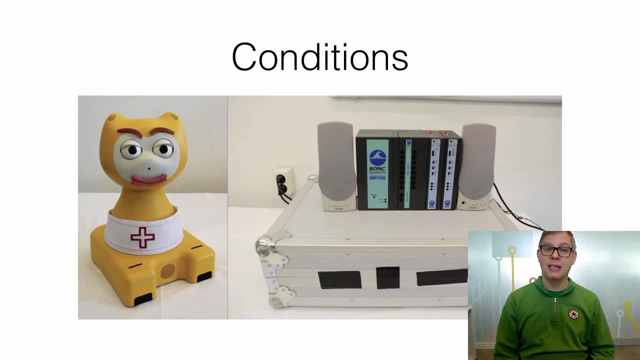 There are quite a few medical examinations that are embarrassing, and people tend to avoid taking these examinations out of embarrassment. They just don't want to do it because it is embarrassing. Now, if robots would do this kind of tests, this might be far less embarrassing and therefore, 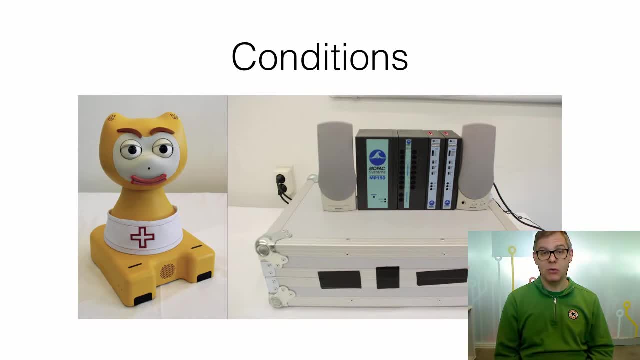 humans might be inclined to attend these critical tests much earlier, which again would help considerably with the diagnosis, or the early diagnosis of some of the problems. So you see here the two conditions where we have a more human-like robot, actually more like a cat-like robot, and something that can only be described as some sort of box with lights and switches. 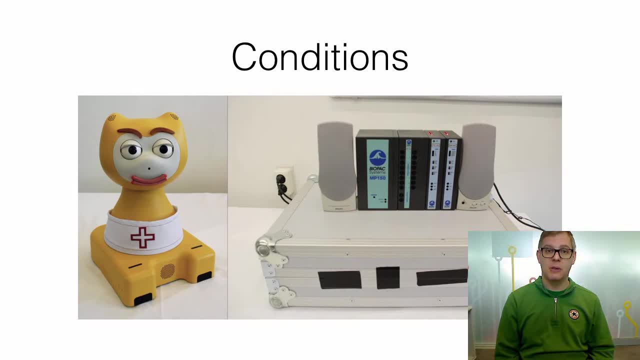 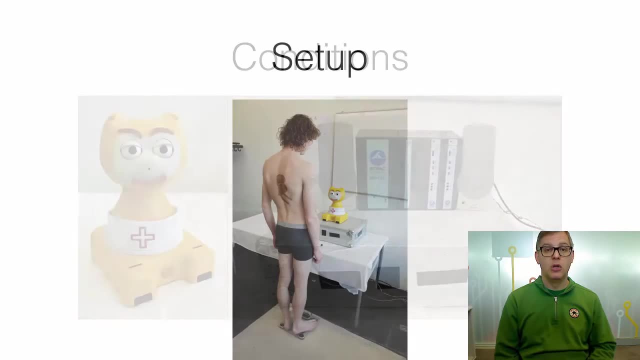 So these were the two conditions we had, where we asked participants to perform, or these kind of two machines would ask the participants to perform an increasing embarrassing examinations, So where this would start with an eye test and we would then ask them, for example, to undress to be able to take an accurate weight measurements and 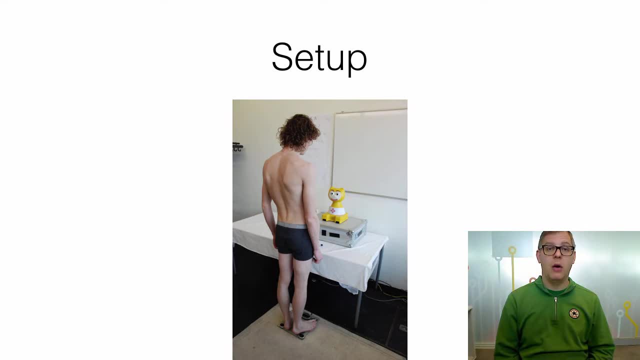 then there were a couple of other tests beyond that, And our question was: well, do people be more embarrassed? and there were two type of embarrassments tests that we did. One of them would, of course, be a questionnaire that we would apply afterwards, but we would also 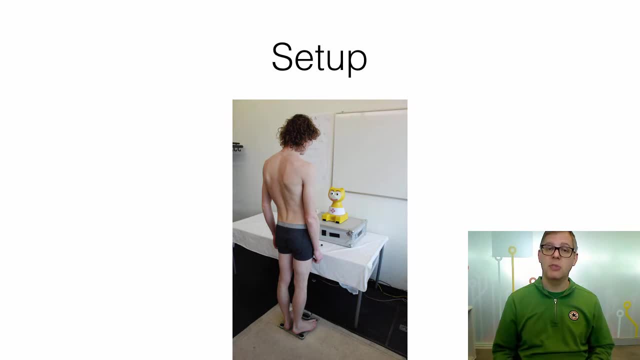 look at the behavior that the people showed. So there's some very typical behaviors that people show when they're embarrassed, like they would like do like this, or they would, you know, hide their face. There are some signals in body language that you can pick up, that clearly. 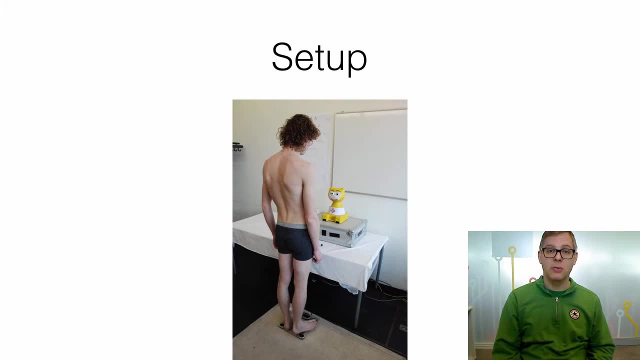 indicate embarrassment and since this whole session was video recorded, we were able to do this And, of course, after the analysis or after the experiment, you know, the participants were fully informed about the intentions of this experiment, since we did had to hide the fact that this was a study about embarrassment. If you run a study on embarrassment, you can't tell them up. 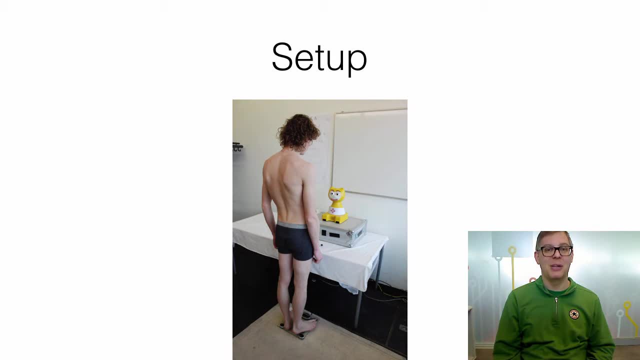 front, because otherwise they know that it's about embarrassment and they will modify their behavior accordingly. So we did have to work with deception and, as it is appropriate, the people were informed about the deception afterwards and we there, of course, were offered to be excluded from the study and all that data being deleted afterwards. 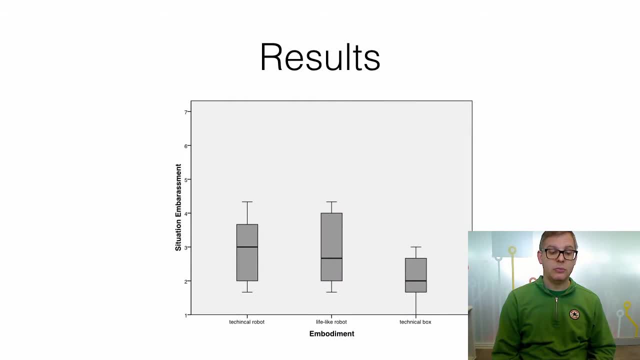 Now what we could sure see is that the people were more embarrassed in front of the robot than compared to when they were dealing just with this technical box, which means that these robots were also perceived as being more anthropomorphic than the box. Now, one of the problems with the study is, of course, that we did not have a chance to include 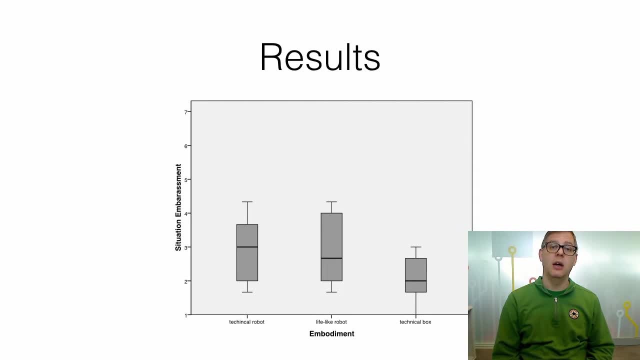 a human condition in it. We did not have a nurse in there in front of which the participants would have to perform these tests, which, of course, would be also very interesting, But nevertheless we could see that, you know, a box was definitely less anthropomorphic than this particular robot. 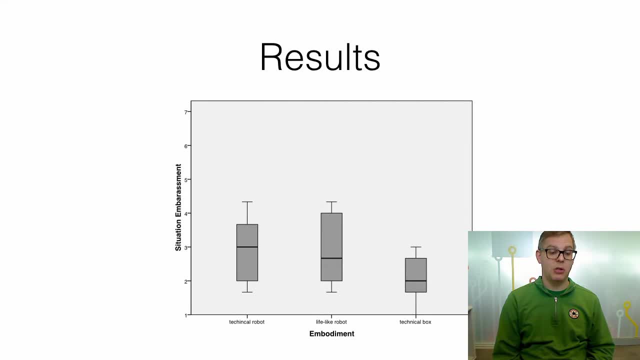 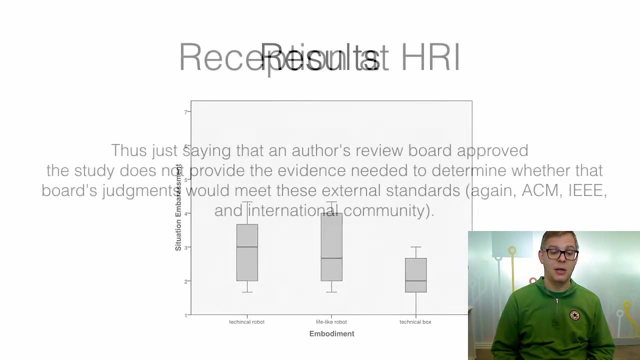 Now, what makes this particular study also very interesting is its reception. We submitted it to a conference And when it came back with reviews and we had a chance also to rebuttal it, one of the biggest concerns that the program committee had was about the ethics of this study, And one of the arguments 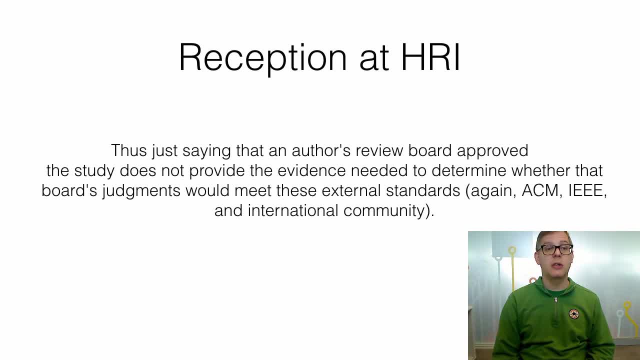 that was brought forward, roughly speaking, is that this study did not comply to the ethical standards of the ACM and or IEEE and would therefore not be suitable for the conference. Now, I got quite furious about that and I actually looked up the ACM code of ethics to see what they actually have. 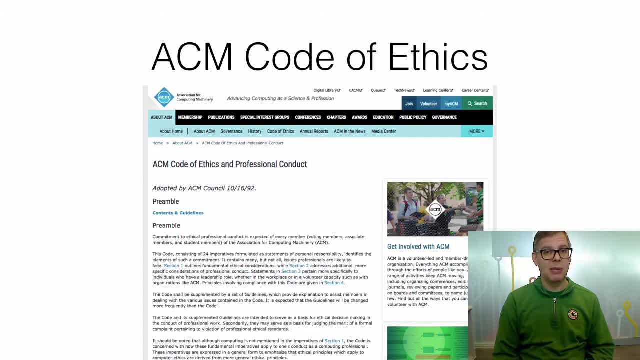 to say about it, And sadly they have got nothing to say about it other than you're not supposed to harm participants in your experiments. The ACM does, for example, explicitly at Laos, investigate in killing people in the form of military research. Now, that is perfectly okay, but there was 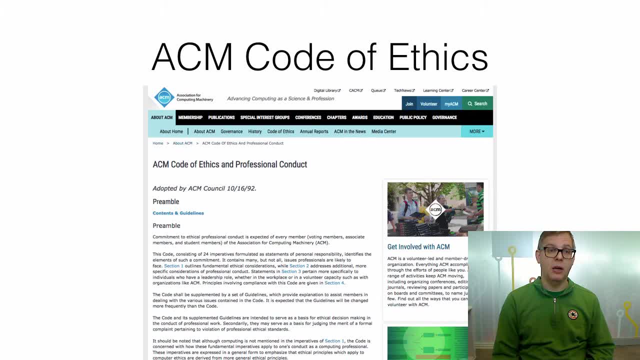 no clear measure of mentioning of anything that you would see, let's say, in an ethical approvals procedure that we have here at the university. that does not exist. So the argument that the conference brought forward at that time was rather shaky. A possible explanation of this is, of course, that the program committee was largely 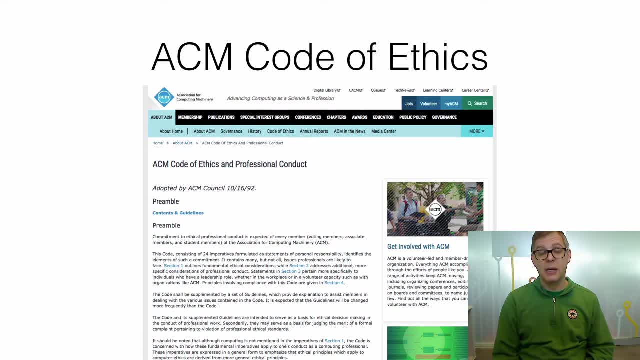 made of researchers from the US, and the US is certainly more conservative when it comes to sexuality. In my perception, it was definitely quite striking how difficult it was to embarrass Dutch students, since this study was done in the Netherlands and they didn't really mind doing any of these tests. 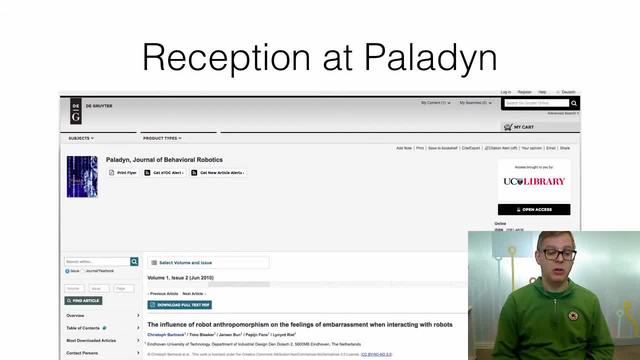 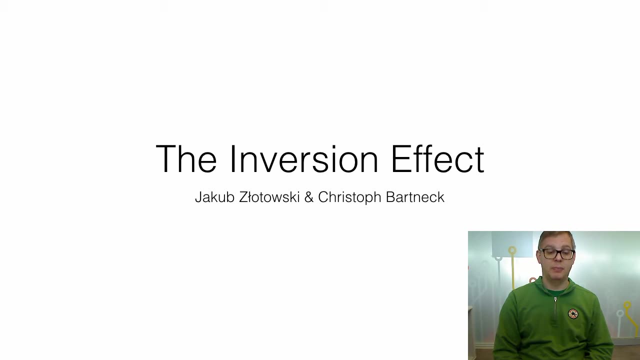 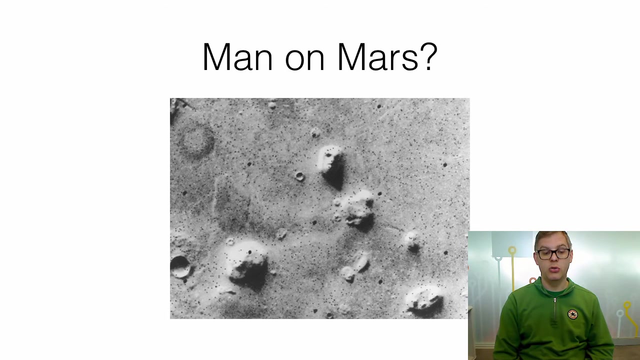 Now. we then went on to submitting this paper to a journal called Paladin, and it was accepted without any ethical concerns. So what we see here is that ethics can be quite relative. Now, another aspect that we were looking at is the inversion effect. Now, when the NASA flew out to Mars in 1976 with this Voyager drone, 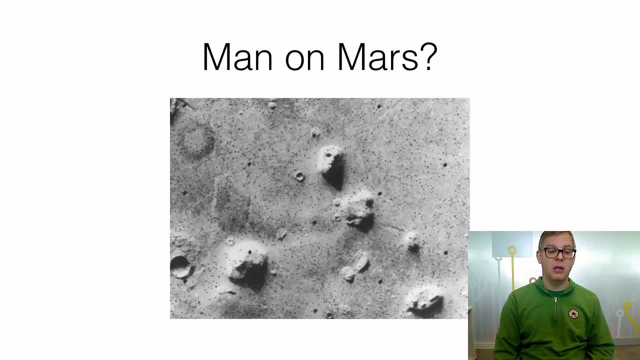 they took this photograph And what you see is there is a rock and it looks like a face And there's been countless rumors and theories about, you know, people living on Mars. So the NASA did, actually felt compelled to when they said: sent their next. 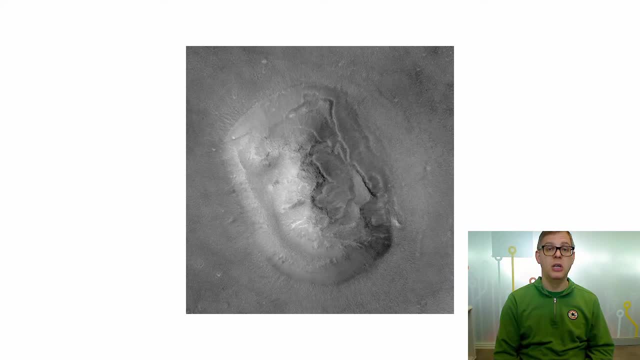 Mars Global Surveyor drone to Mars in 2001 to take another photograph of this exact rock, And what you see now, with the different light conditionings and a much higher resolution, is that it is not a face. it is really just a rock. Now, the interesting thing here is that we have 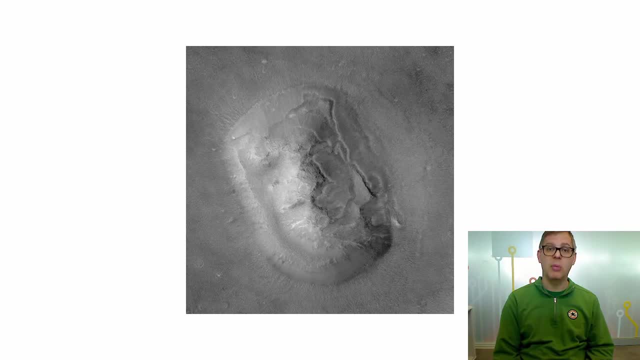 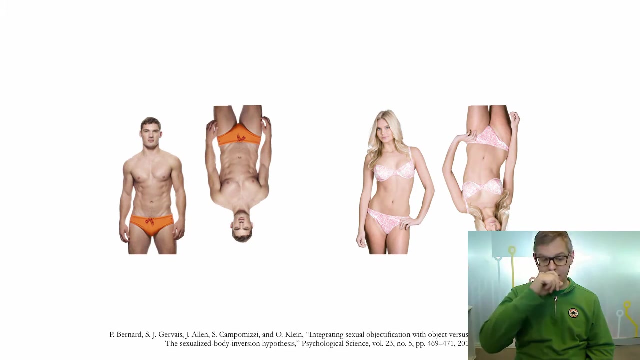 this built-in mechanism of looking at our environment and interpreting faces and anthropomorphic features into it. Now this can become quite interesting. For example, we encountered this very interesting study where, when you do take a human body and you present it just normally, we can recognize it relatively. 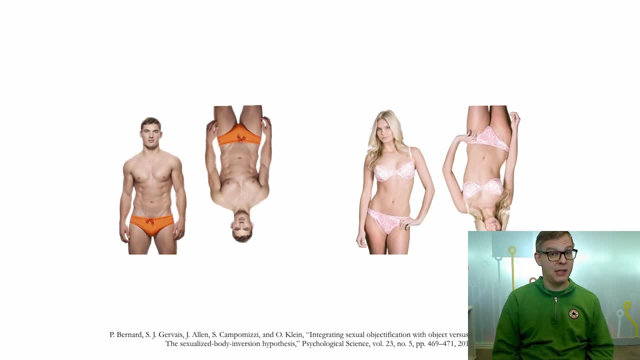 easily. But when you take this body and you turn it upside down and you ask them people to recognize this body or compare it to another, to say if it's the same or different, the task becomes considerably more difficult. It takes people much more time to do this. 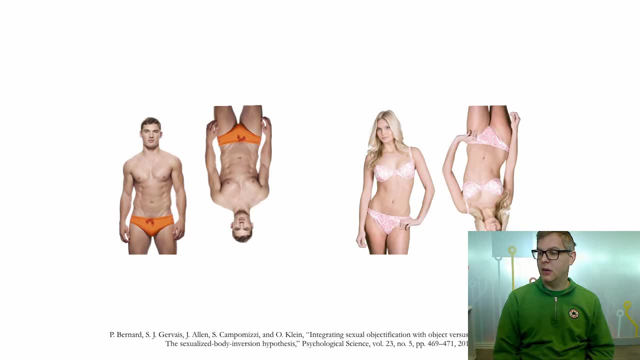 Now in this study from Bernard and Gervais, Allen and Campuzzi and Klein, they went a step further and put gender into the equation, So they had this sexualized bodies here, So essentially bodies or people just in the underwear and run this kind of test. 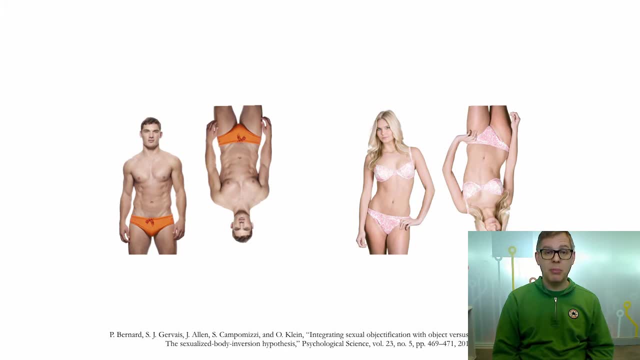 And what they found is that for the male body it was indeed harder participants to recognize the body, But for the female body that was not the case. The female body was perceived similar to how we perceive objects, And they were making the claim that 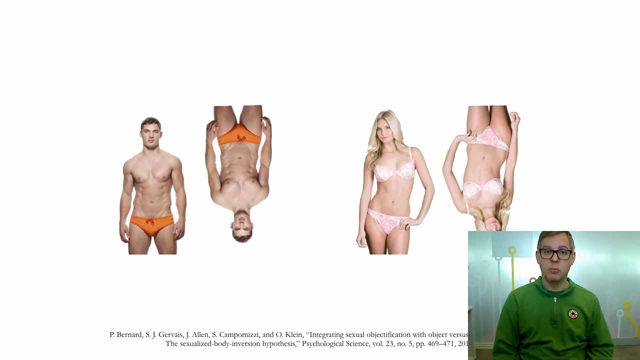 this is an indication for how the female body would be perceived as being objectified. Now, that kind of triggered us because we thought: well, if it is possible to objectify, to dehumanize a human body, can this test then also be used the other way around? Can we use this kind of test? 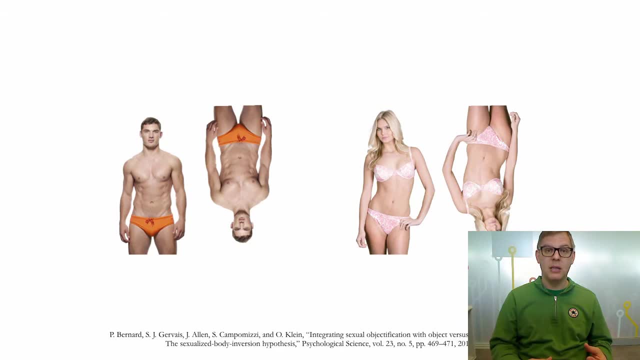 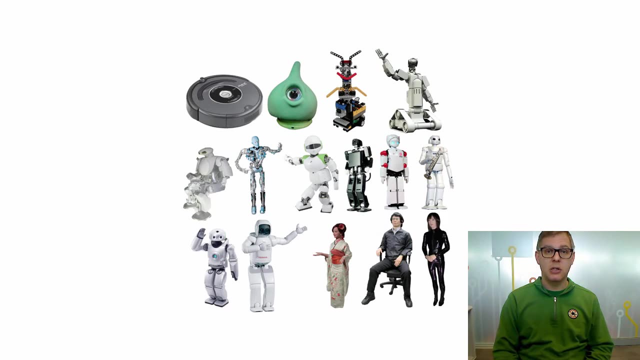 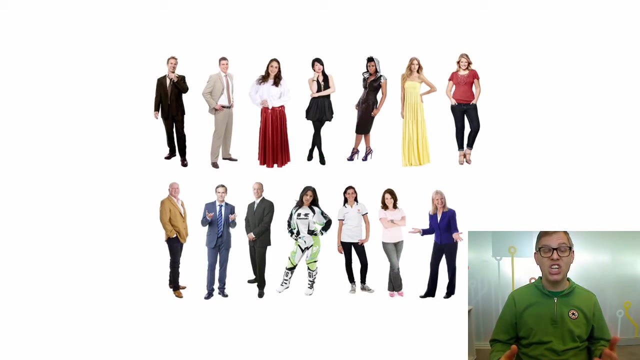 to see whether robots are being humanized. Now we took a couple of robots And you see here a selection of them, because we wanted to cover a wide range of robots And in our case we did not particularly look at gender. So we're not interested in male-female bodies, So we just 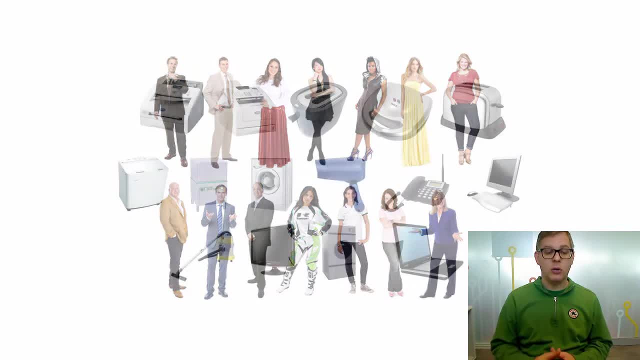 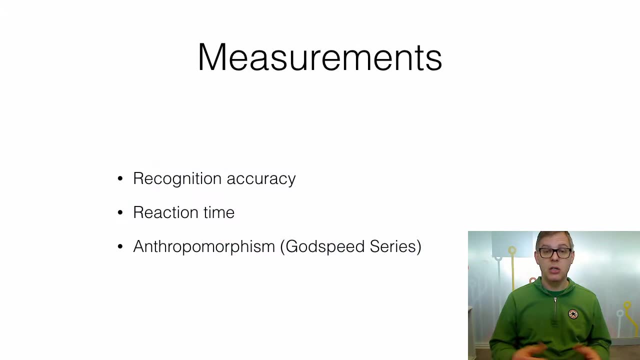 took well-dressed robots And we did not look at gender. So we did not look at gender. So we people And we also included objects, everyday objects, And for the measurements we took the recognition accuracy so whether they would actually identify two, for example, two pictures. 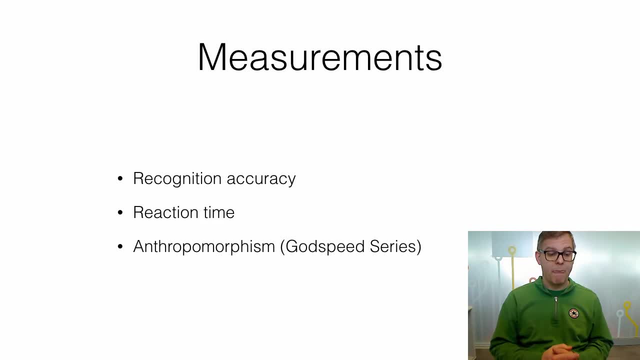 of a toaster to be the same or not, how long it took them, And we also applied a more traditional questionnaire on anthropomorphism. Now, it's important to say that the exposure time that we had was very short, So that was actually on a subconscious level. So you would see first an 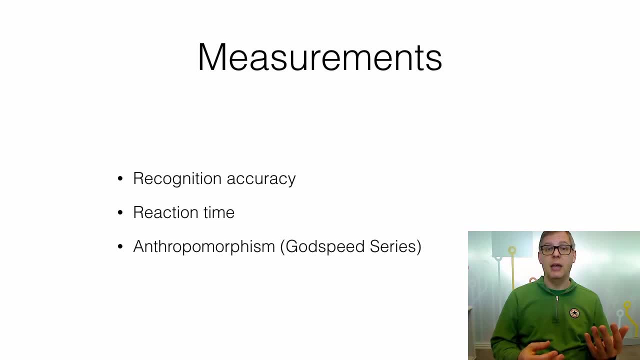 image, let's say, of a toaster, and then the screen goes blank, And then, just for a few milliseconds, you see another picture, And it was either the toaster or not, or it was, you know, manipulated, But it was so short that it could not enter your consciousness. you essentially had to make a 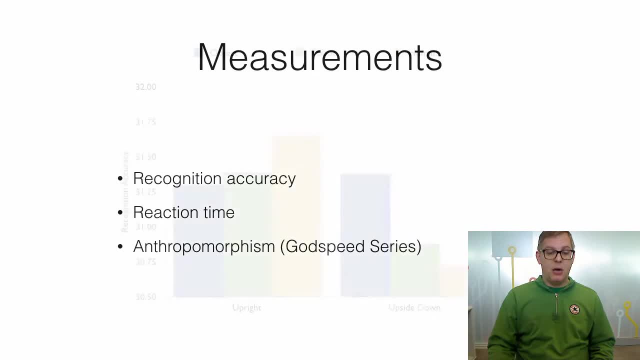 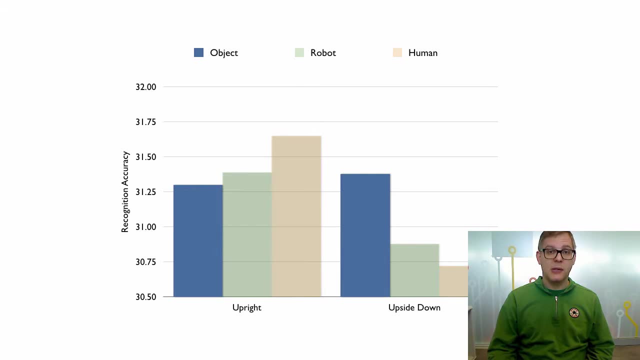 subconscious decision here. Now, the results were of course rather interesting, And when we first look at the objects, we could clearly see that there was no difference in the reaction time for robots. So it was just an authority recognition accuracy. So it was just as easy, or as difficult, as you might see. 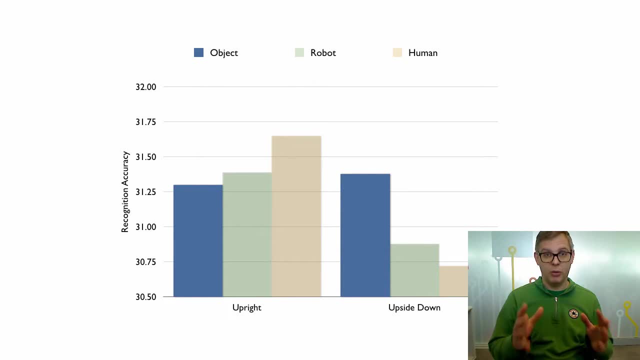 it for objects to be recognized whether they were presented just upright or upside down. Now, when we look at robots, we do see a significant difference. So when the robot was being presented upside down, the recognition accuracy went down significantly And, as expected, also for 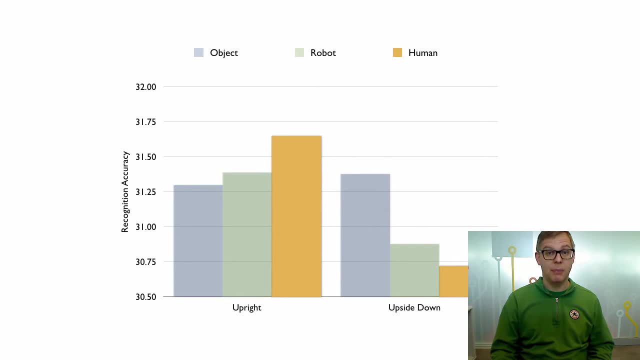 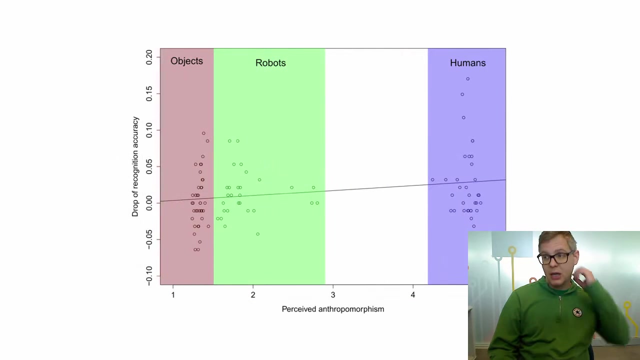 humans, the recognition accuracy went down significantly. So the inversion effect does work for as a measurement tool for measuring anthropomorphism. However, there are other problems with it, And that is explanatory power. So when we looked at the, when we plotted the recognition accuracy, the drop in 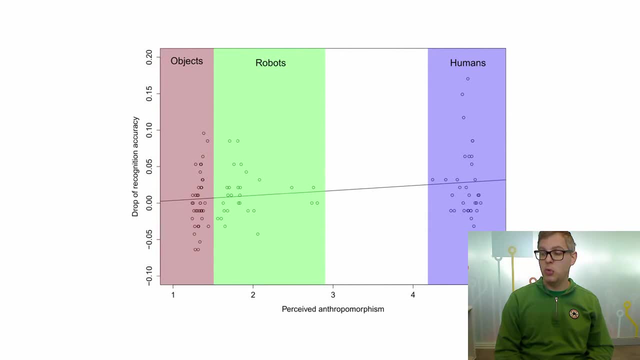 recognition accuracy in this inversion effect to the perceived anthropomorphism. based on the Godspeed questionnaire series, we could see that the explanatory power of the questionnaire was so much higher. It also became clear that we have a large gap there where all the robots 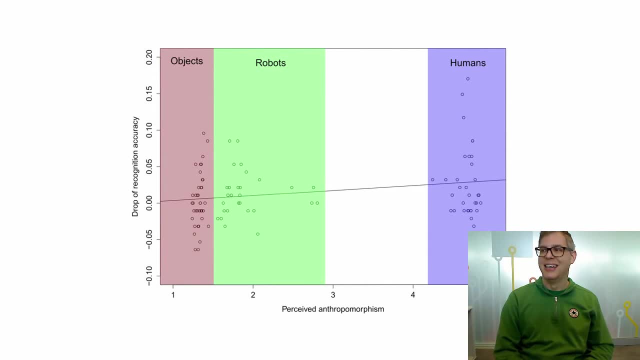 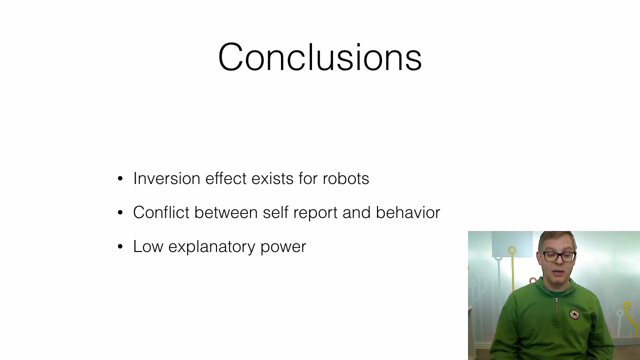 were actually clustered more towards the robot, to the what's the objects, then, rather to the humans. So, overall, the questionnaire still did seem to be the better choice for measuring anthropomorphism, And one of the biggest problem, of course, is that the low explanatory power, that the inversion, 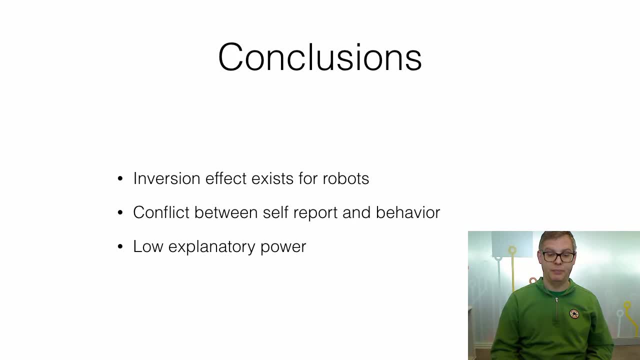 effect has, despite the fact that, in principle, it does work. Now, when we have anthropomorphism, one of the things we wonder, of course, is that: well, if they do anthropomorphize robots, what consequences does that have on how we interact with them? 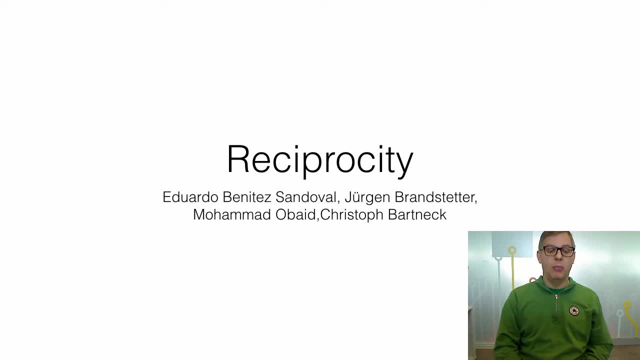 So one of the studies we did was on reciprocity. So reciprocity is the idea of it's an old, essentially social convention that if you help me, I help you all the other way around. And we ran an experiment that was based on, you know, the participants either playing with a human agent. 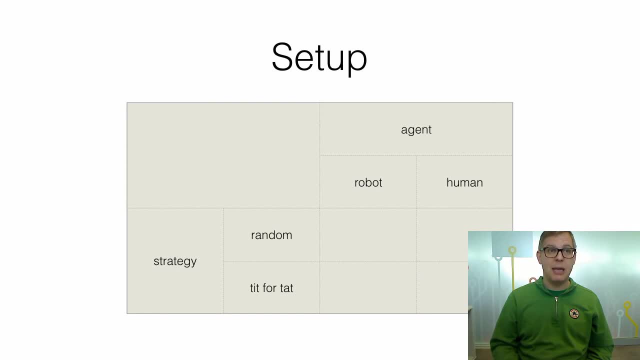 or with a robot, And they would play a certain game which was called the Prisoner's Dilemma game, which is a very well documented interaction that comes out of the field of game theory, And in there people have the opportunity to either collaborate or defect, And they have to make this. 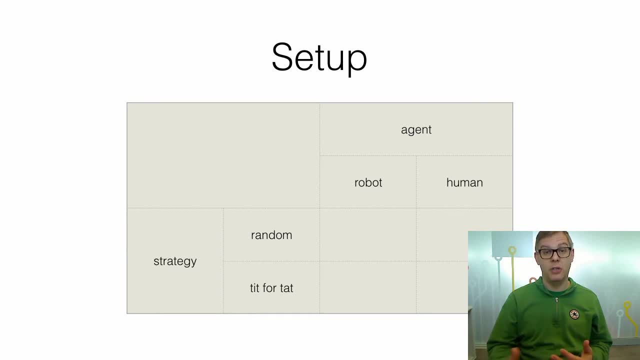 decision independently of each other and without the knowledge of each other, And depending on the of the outcome, they either get rewards or punishment. So, for example, if both of them decide to collaborate, they get the highest reward. If one of them decides to collaborate and the other one decides to defect, 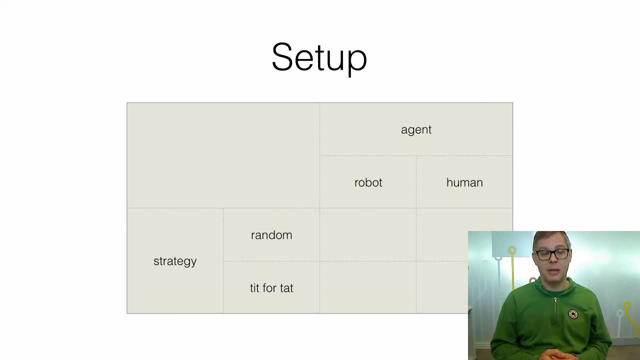 then the person that collaborated get actually the biggest penalty. Now this is a very well documented game, And the robots would actually use- or actually the agent itself would use- two different strategies in this interaction. Either they would act randomly or they would utilize the tit for tat. 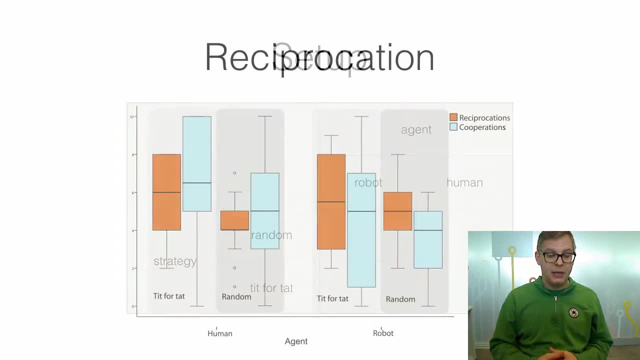 strategy And what we could find is that there was no difference in reciprocations, But reciprocation is not the same as collaboration, So there was actually significant less cooperation with the robots compared to the human agent, And there was also more collaboration and reciprocation in the 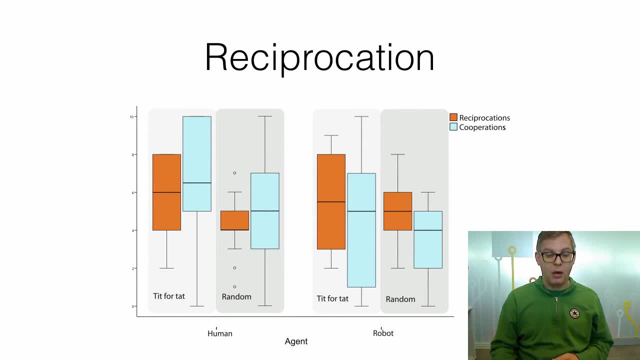 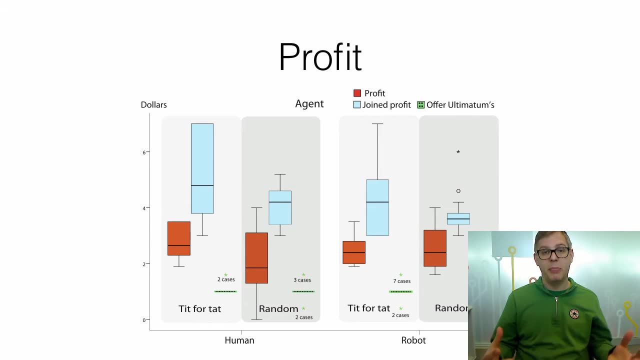 tit for tat condition compared to the random condition. What is also interesting is that the joint profit is in the human condition. So, when you see it from a bigger picture, what you of course want to get out of this interaction is that both the human and 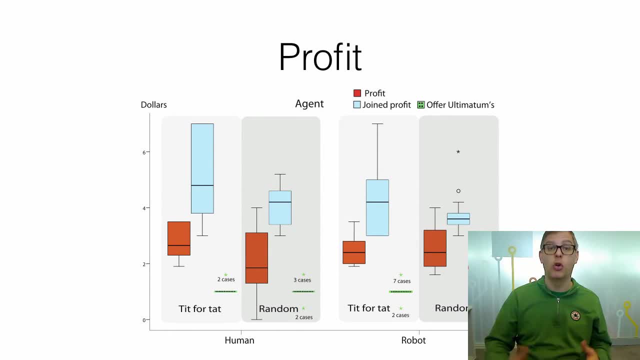 the agent as a participant and the agent in the human robot together actually get the biggest benefit, and this was actually achieved much more with human being an agent than rather being a robot. Now, this was, of course, a first step in an interesting direction, but this kind of exchange and reciprocation can of. 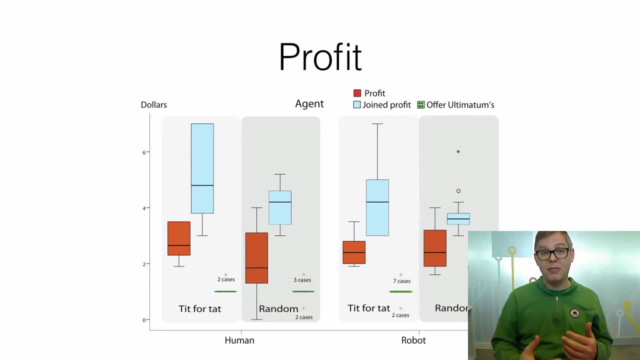 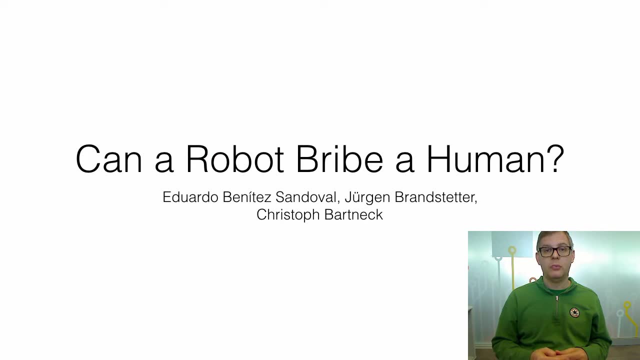 course go also to the next step, and that is the exchange of favor- can actually become criminal, and that's when we talk about bribing. So if you know- let's say you offer me $100 in exchange for getting an A- then that would be clearly. 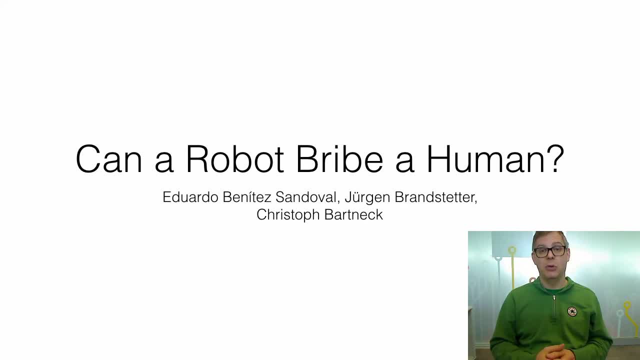 considered violation of rules and it would be considered a bribe, and that is unacceptable. but the borderline between what is an exchange of favor towards what is a bribe is not so clearly defined. But let me show you an example of the problems that can occur. Now, here we've got a robot called HitchBot and 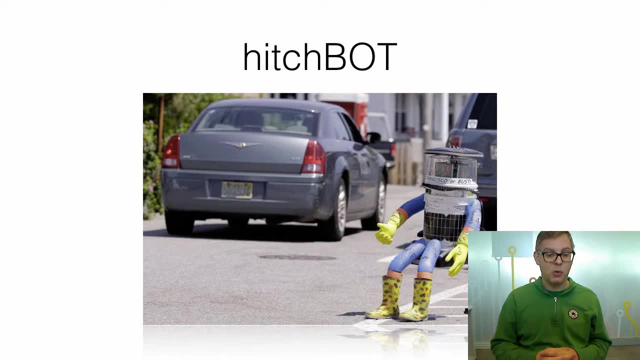 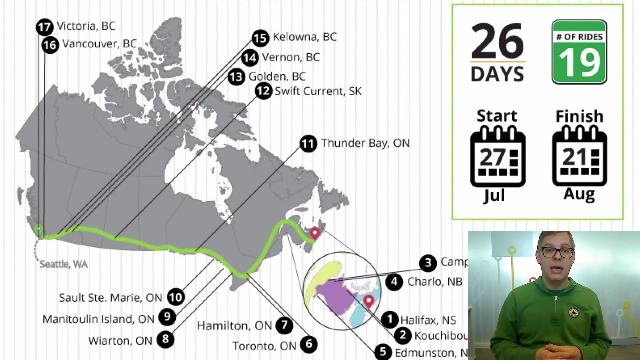 HitchBot was set up as a hitchhiking robot, so it would be set up next to the street, and was trying to essentially cross the continent in Canada, and it did so. It took it 26 days to go from one side of the coast to the other, and it was. 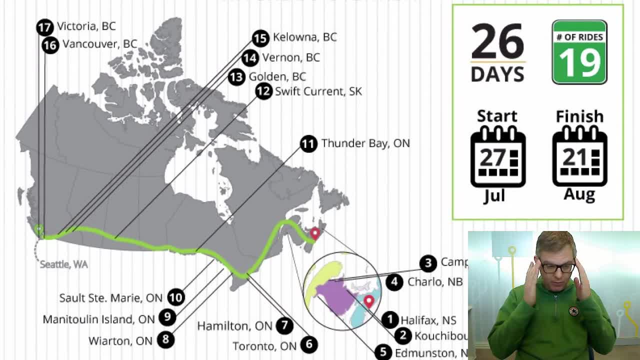 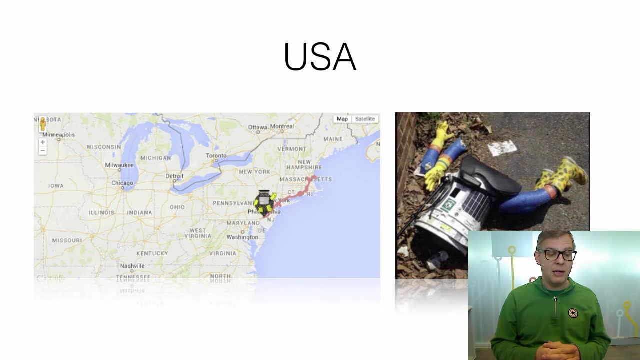 purely, of course, based on the goodness of the people that decided to take it along, and it all worked very well. Now, sometime later, the same researchers tried to do the same experiment in the US, but unfortunately, this robot barely made it, and barely made it, it was actually destroyed very quickly after. 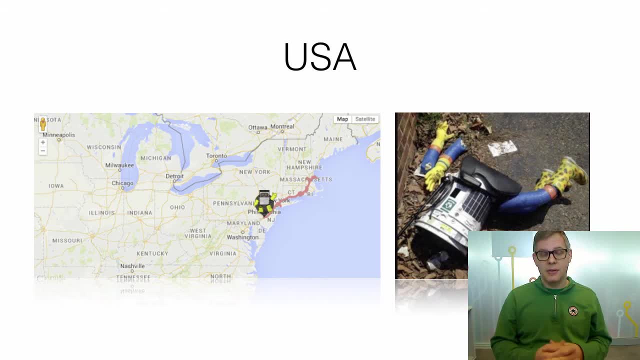 its start. Now, the reason why I'm bringing this up is that this was a very one directional interaction. it was not really a reciprocation. The robot could not really offer anything in return to the kindness of the people to carry it along, other than possibly getting a bit. 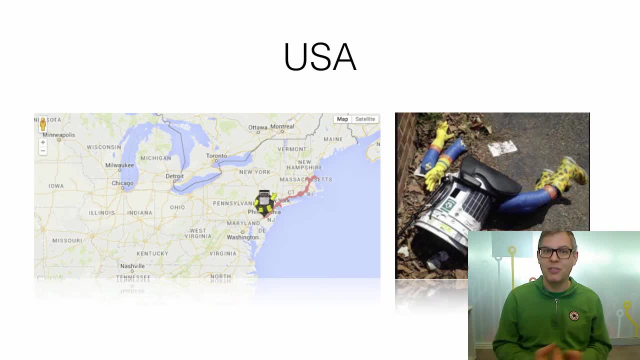 of public relations or you know, they could, you know, shoot selfies with this robot and, you know, have participate in a bit of fun, but the robot wasn't actually able to do anything for for the robot. So it is very important that the robot is able to act and to be able to have something to exchange in order to have a 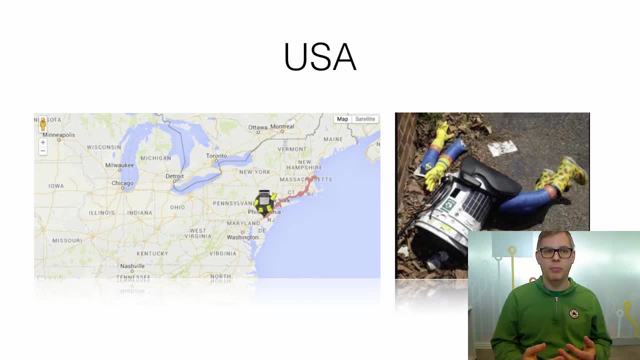 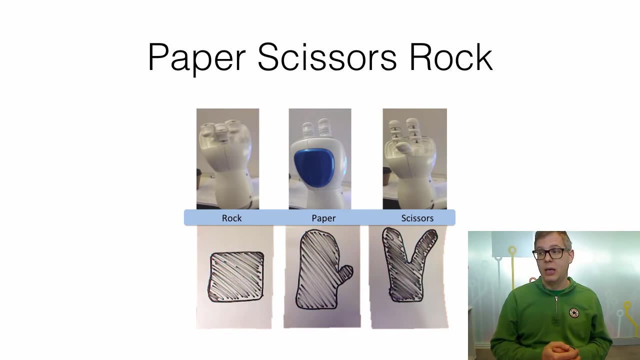 very fruitful and beneficial interaction with humans. Now we run a an experiment again with a robot where the robot would play paper scissor rock and unfortunately our robots are a little bit more simple than humans, so we have to devise different kind of gestures, since the robots we have only has three. 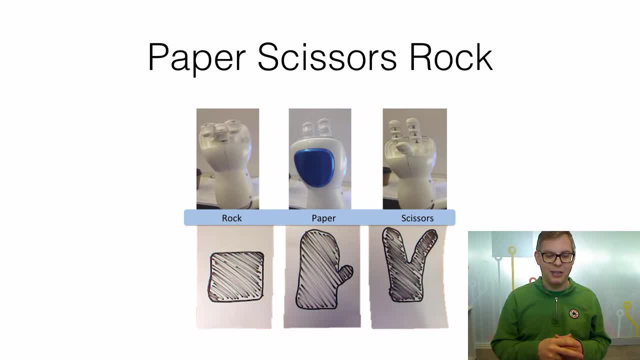 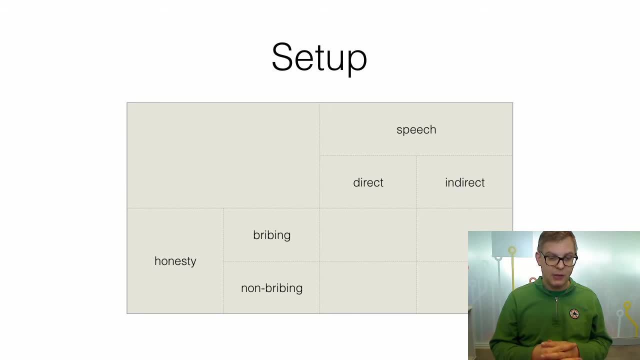 fingers. so slight modifications to the, to the symbols used, but very easy to learn. and the setup was that either the robot would cheat during the interaction or it would be honest and it would either use a direct speech or indirect speech. So let me give you an example. 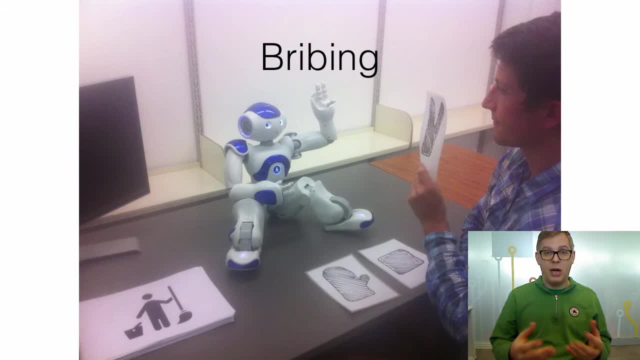 In the case of the bribing robot, the participant, the robot would actually, you know, after, let's say, the robot won, change its setting or change its choice so that the human would win. So it would actively try to lose in order to give favor to the human. and when it did that, it would either use direct or 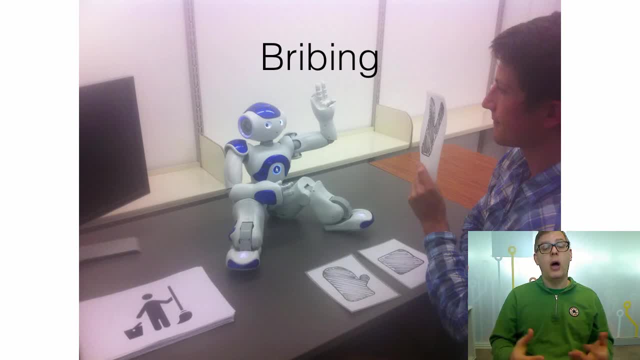 indirect speech. So it would either use direct or indirect speech. So it would say: oh. in the direct speech it would say: oh, I will need your help later, you know. or in the indirect speech it would say: oh, please enjoy, you know, this extra win. you know, maybe you can be of helpful to me somewhere in the future. Now the 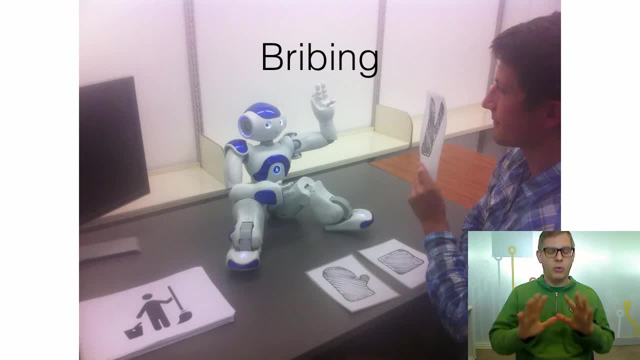 interesting thing is that only three out of sixty participants- oh, hold on a second, I'm getting ahead of myself- after the study. so after this interaction with paper scissor rock, there was a second phase in this experiment, where the participants, the robot- would actually ask help of the participant and the 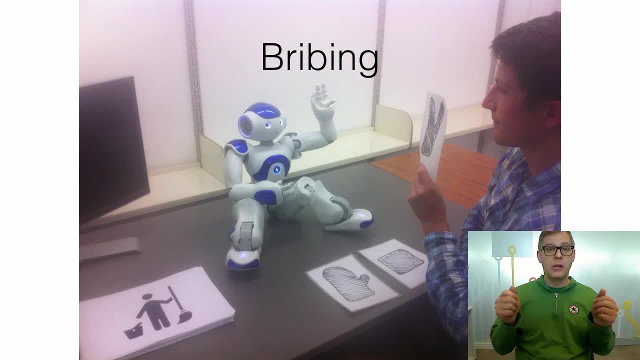 tasks that the robot asked for was to show it an icon. as you can see here on the left, there's an icon on the left, a person with a mop, possibly a janitor, and the task was that the participant had to show this image to the robot and tell. 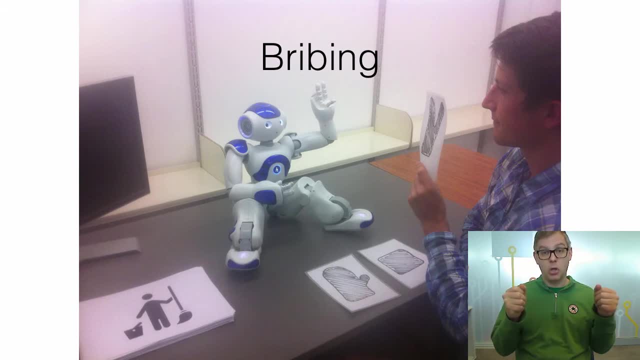 the robot what the picture actually shows. So they would have to say: this is a janitor. This was an open-ended task, so the participants could do this as long as they want. and there was, you know, they could stop whenever they wanted to and of course, our hope was that you know if the robot actually you 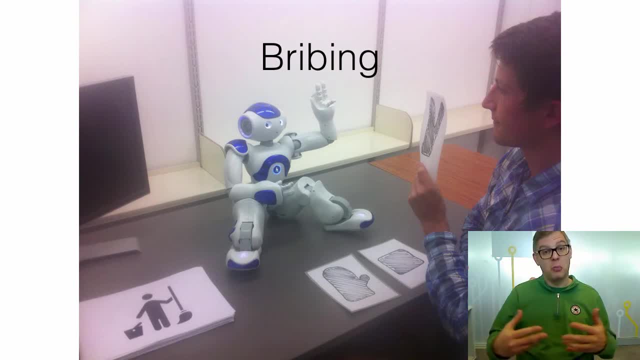 know bribed or let's say the participants- or lost on purpose, that the participant then would feel more obliged to actually help the robot. Now, only three out of sixty participants did not decide or decided not to help the robot at all. All other participants decided to go into the second phase, despite the fact that they it was. 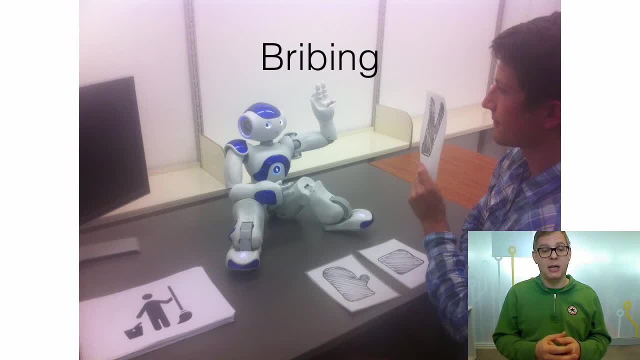 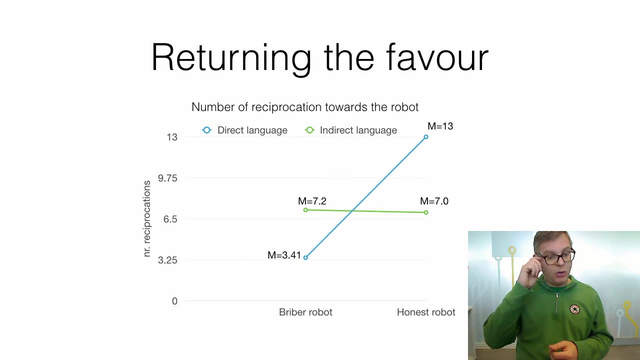 not, it was completely voluntary. they. they could have just not do it and there was no penalty for it. so that was a good sign that they actually participated. But what we also saw was a very strong interaction effect. that means for the bribing robot it did actually matter whether they used an 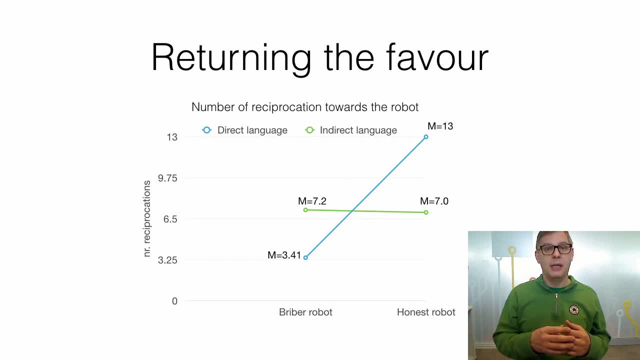 indirect language or not, But for the honest robot it did not matter. So the number of reciprocations was actually state stable for the indirect language, or let's say, may put this way, the honest robot, actually that use direct language received most reciprocations, which means 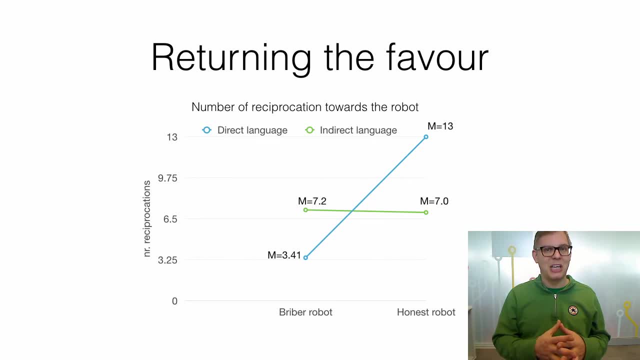 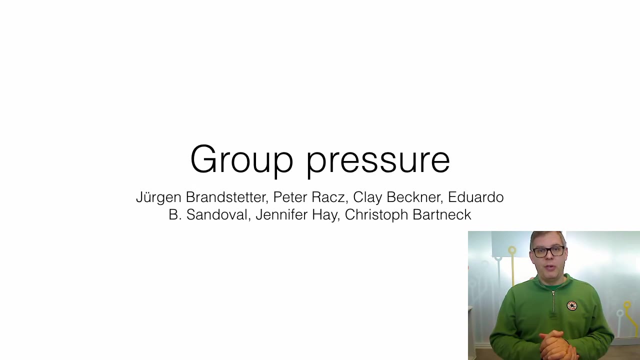 that, despite our initial idea that actually, you know, a bribing robot might be useful, This study actually shows that an honest robot that uses direct language is the most successful robot. Now, since you all, or some of you, are familiar with psychology, you might, of course, very well be aware of the ash. 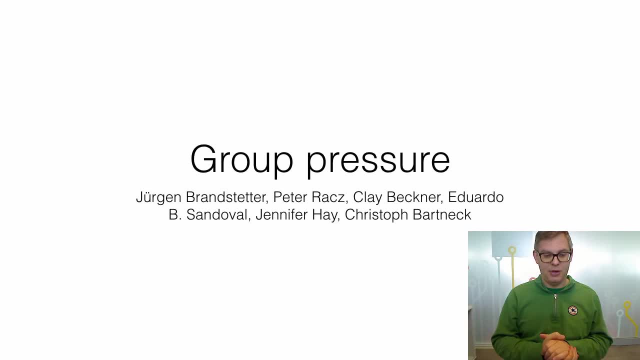 experiments, But for those of you who are not, I will get to you In a second. Now, this experiment was about group pressure Now, already today. I mean, we have only very few robots around. we have some robots that clean the floors. 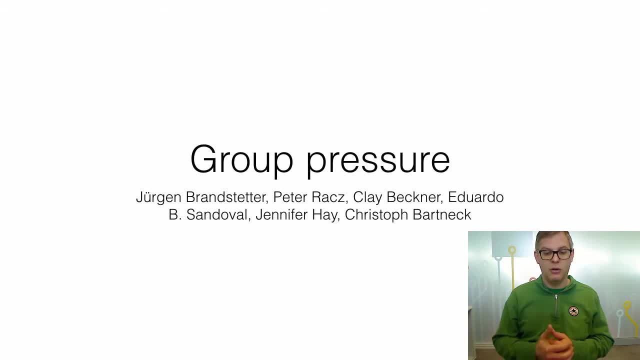 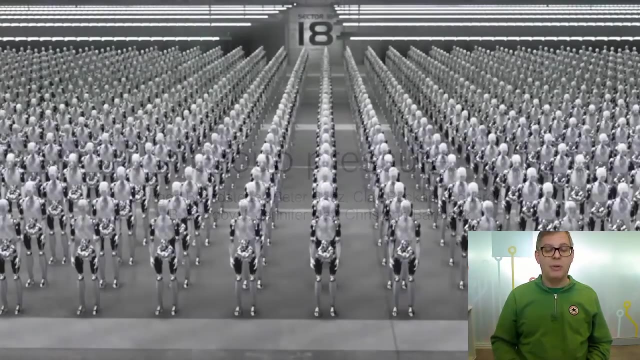 we've got some robots that you know do all on, And of course we have quite a few robots in the industrial area, where they are used in manufacturing, But still their numbers is quite low, particularly in the private environment. But what happens if there are more robots than humans on the 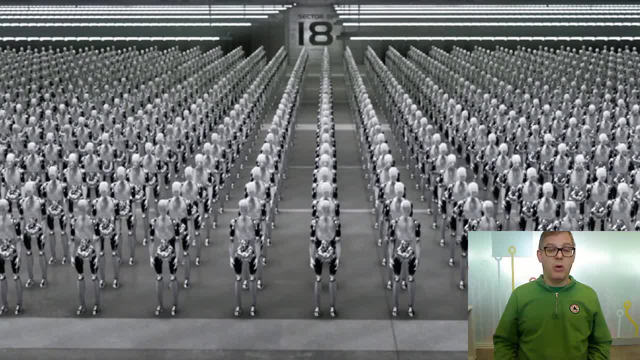 planet. Now Isaac Asimov actually envisioned that maybe in the future we have a ratio of 20,000 robots for every human, And already today we have more telephones or smartphones on the planet than people. So we are getting there. And the question: 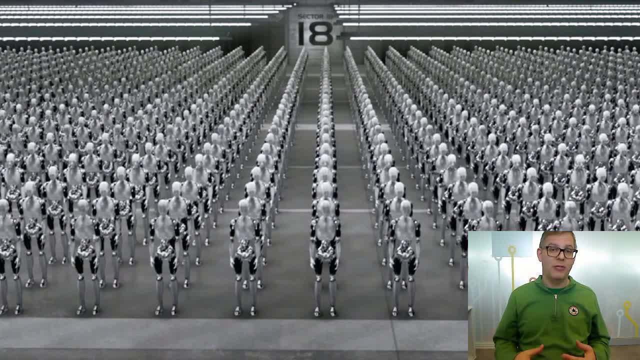 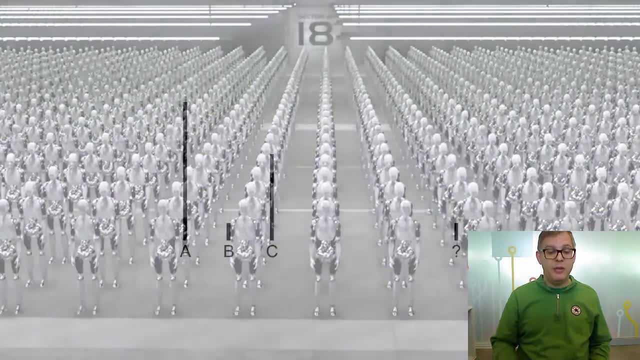 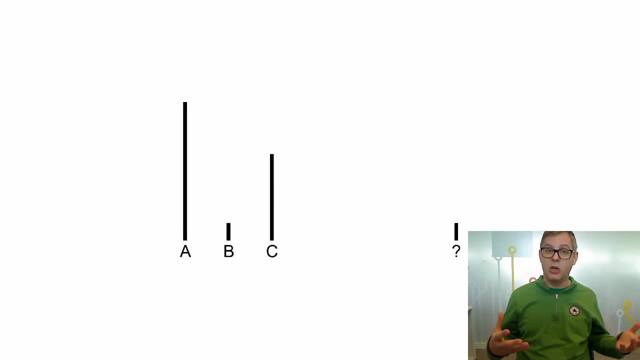 of course, is when we have, you know, a majority of robots. can these robots execute any kind of group pressure on us? Now, the very famous ash experiment was set up in a way that participants would come into the room and they would sit down and they would be presented. 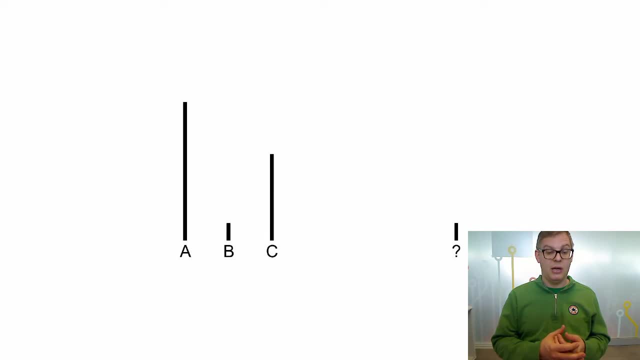 with a slide like this, And each of them had to add what have to give the answer to the fourth line here, the mark with a question mark, To which is this equivalent to either A, B or C? Now, in this case, 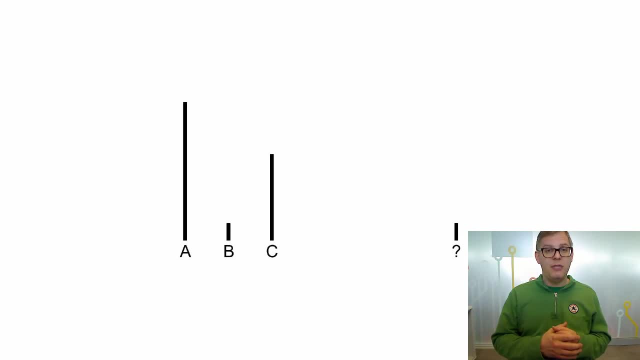 of course, the right answer would be B. However, the experiment was very interesting in the sense that three of the participants were actually actors and only one of the participants was an actual participant, And the three actors would give a consistent wrong answer. So they would. 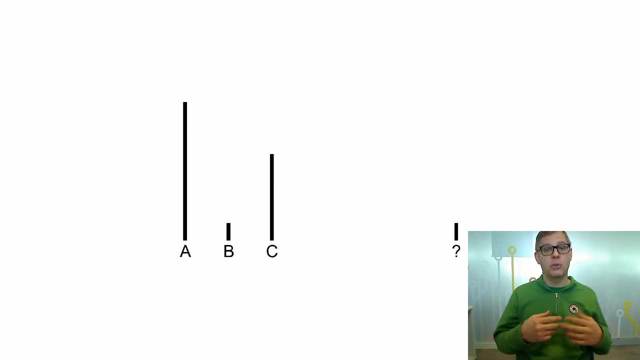 all say, for example, C, And then the question was: how much does that actually influence The unknowing participant? would they actually change their mind from B to C? And what ash could show is that this actually happens, and it happens even stronger the more ambiguous the lines are. So in 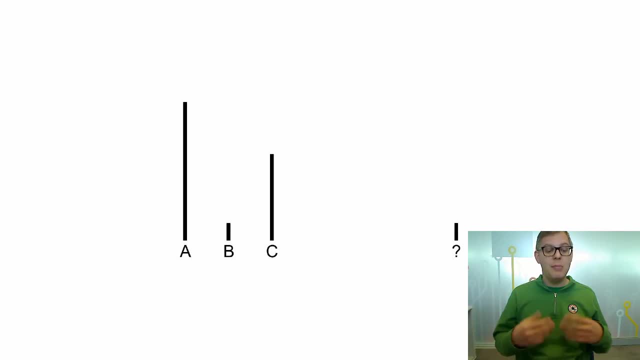 this case it is actually very clear that B is different from C. but if we imagine B to be almost the same as C and the line with question mark also be equivalent to B, we could see why people might actually think like. 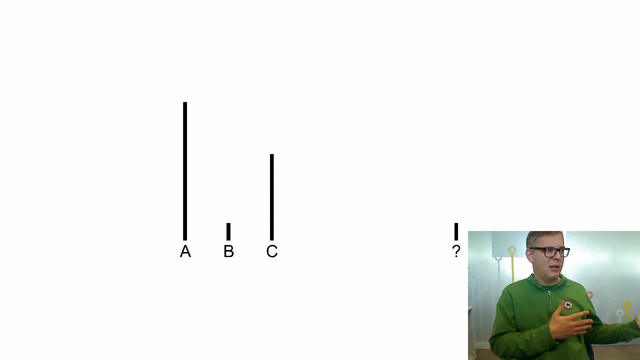 oh well, you know, all these four people think it is that, so you know, well, they must be right. maybe there's something wrong with me now. we use the same methodology, but we replaced the human actors in this experiment with robots, so we would have four robots and one human participant. 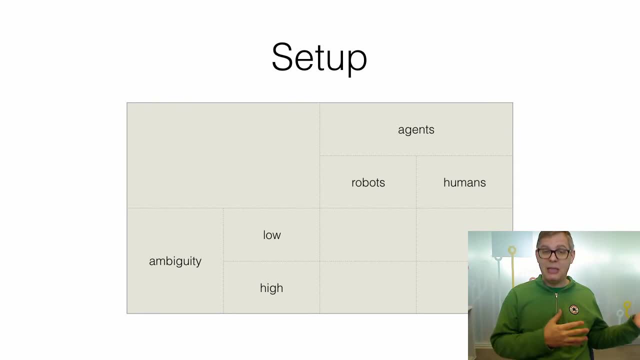 but at the same time, we also replicated ash's experiment, where we also had a condition where we actually had four humans and actors and one actual participant that didn't know, and what we varied also is the ambiguity. so either the lines were very close to each other, 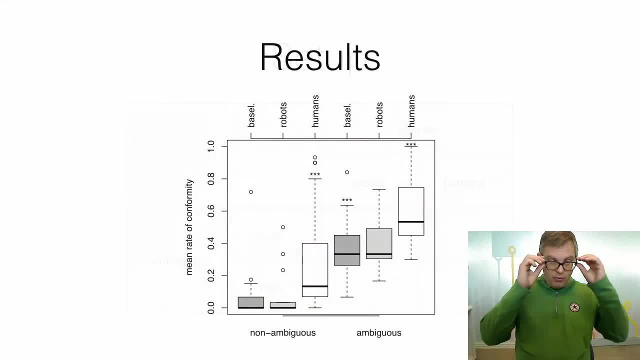 or they were not, and the results show that ambiguity had a clear effect on the result. so the more ambiguous the lines are, the more likely the participant was to agree with the wrong judgments of the other four. now, the agent, however, did not have a significant influence, so 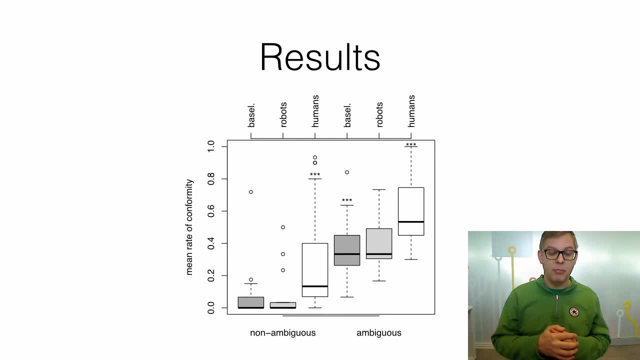 the robots actually do have only the possibility to influence the judgment of the participant in the very ambiguous task, but still it is possible. so while the persuasive power that robots have is below that of humans, they still have the possibility of influencing the judgment of the participant. they still do have some persuasive power. and now we only used four very small robots. 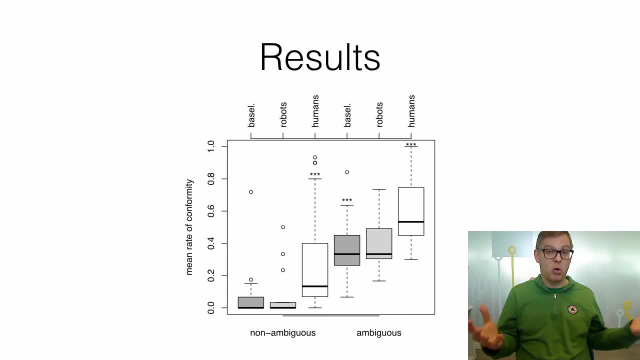 and if you imagine, you have 20 life-sized robots, maybe robots that are like these androids i showed before, indistinguishable or nearly indistinguishable from humans. this kind of behavior might change dramatically now that, since we were kind of interested in persuasion, we then took it to the next level, and that is. 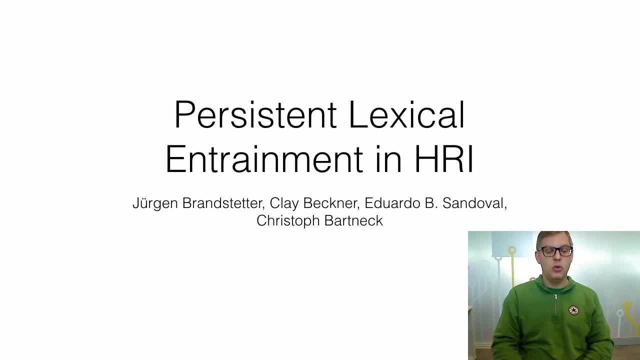 well, maybe what we can do is actually change how people use language. so, for example, if you have, we use the word cup or muck. these are synonyms and you know some people use the one and others use the others. so the question is, when, let's say i have a preference for saying muck, can i be made? 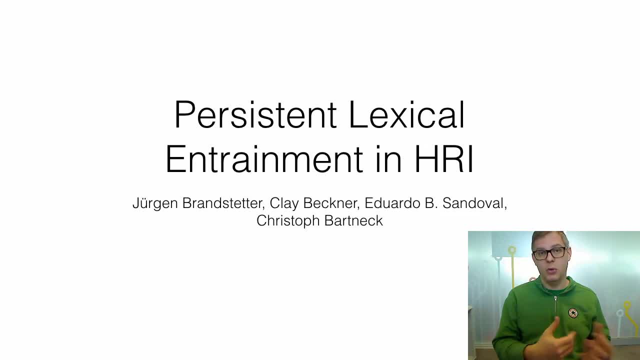 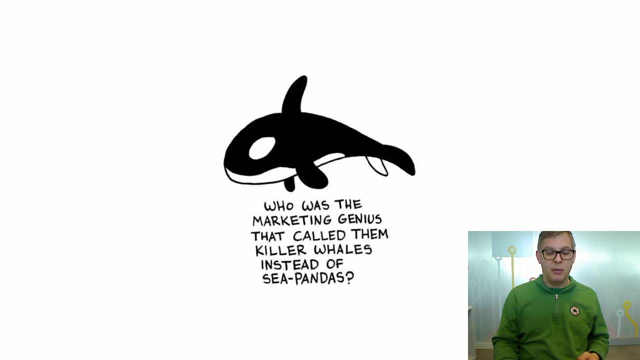 to change my behavior to using the word cup. now, this is, of course, something that you might find is quite trivial, but, however, in public relations, this is actually becoming very, very important. so this is a little cartoon that i found. who was the marketing genius that called them killer whales? 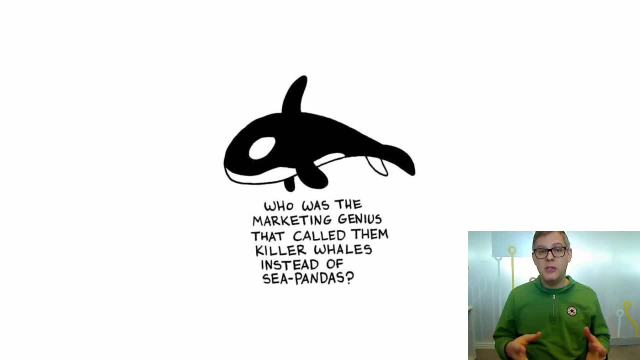 instead of sea pandas. so what you see is that how you call things has an impact on your behavior, and how you think about things has a major effect on how you think about it. so, therefore, the choice of words that you use has a major impact on what people think about certain concepts and what 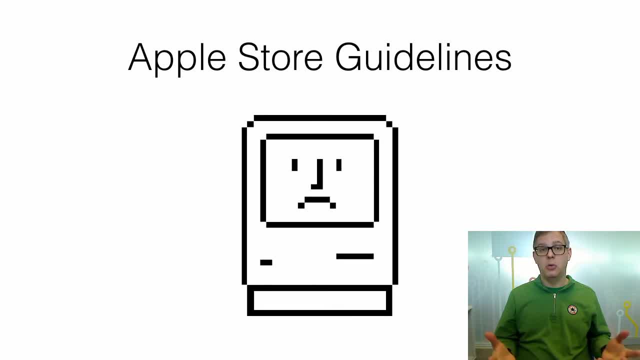 attitude they have to it. so, for example, if you go to an apple store- and unfortunately we do not really have an apple store, an authentic apple store in new zealand- but if you go to the us, they have some shop guidelines. there are clear indications about what the um employees of the shops are supposed to say and 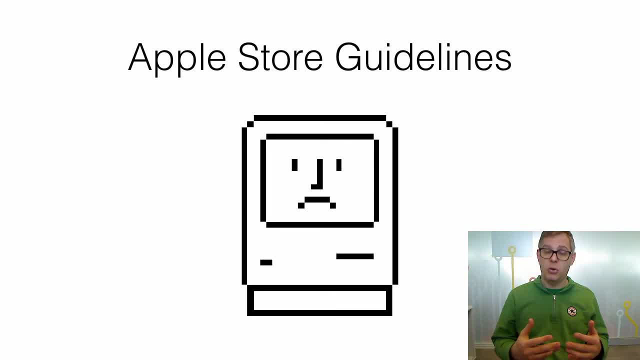 whatnot. so, for example, they are not allowed or not allowed. we're not supposed to say that your mac crashed. what they're supposed to say is that your mac stopped responding. and you see that how this, through these kind of changes in language, you can actually change the attitude, that 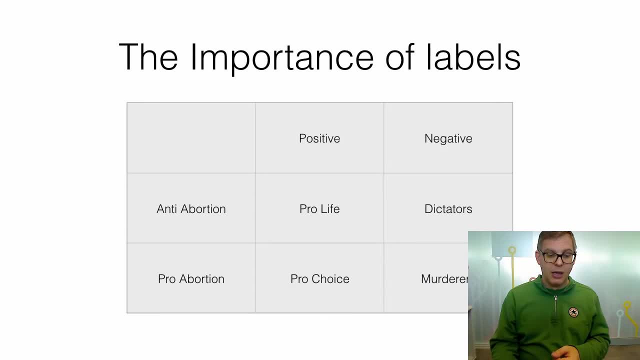 people have towards the product. now, we didn't um. well, if you take this even further now, um, you know, again, this is just marketing. but if we look at this, uh, anti-abortion or the, the discussion about abortion, you know it gets of course much more, let's say, um important. so the anti-abortion of 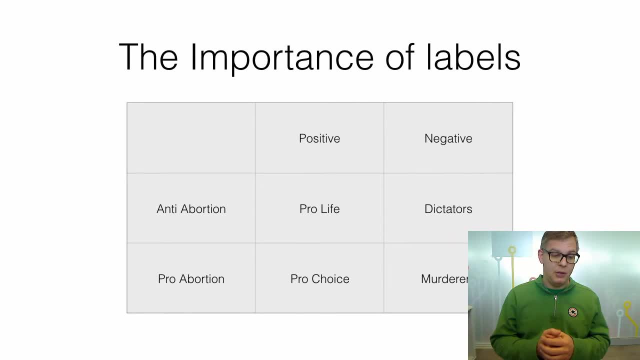 course, uh faction call themselves pro-life and the pro-abortion people go by pro-choice- and of course they could have also called themselves pro-abortion. but what they really want to say is, well, you know, pro-choice, because who could possibly be against people having a choice? um, and the same thing holds true for the anti-abortion people. how? 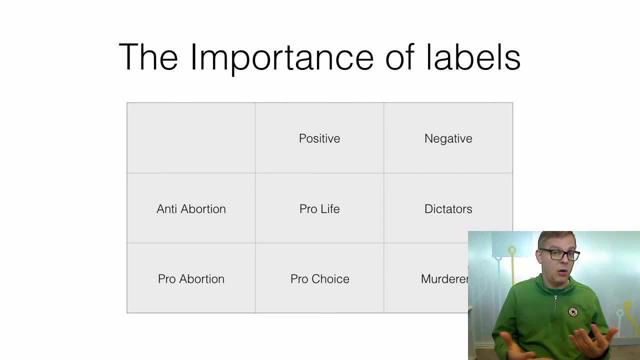 can you possibly be against life and if you, you know, turn this in a negative way, you know you could actually call the anti-abortion people pro-life and the pro-abortion people go by pro-choice and the pro-abortion people murderers. so you see how you, what labels you use, can be really, really. 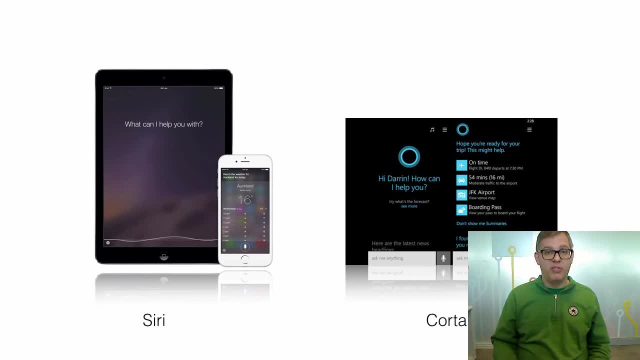 important and, as i mentioned before, we already have more phones on the planet than people, and these phones and computers these days have the ability to recognize our speech and to reply in speech as well. so apple has got siri, microsoft has got container and um, google also has a speech technology and um. and then the question comes: what? 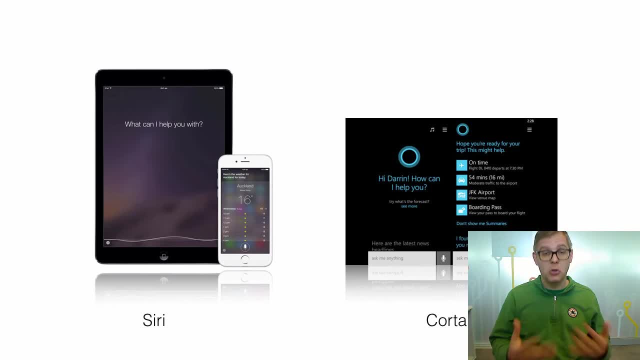 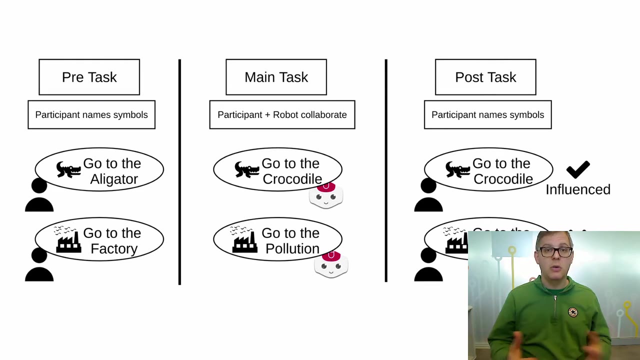 labels? what words do these machines use to talk to us? and, furthermore, who is controlling the vocabulary that these machines use? now we did a test where we first looked at participants in a pre-test to see, well, what is the, let's say, normal label that this participant would use. so 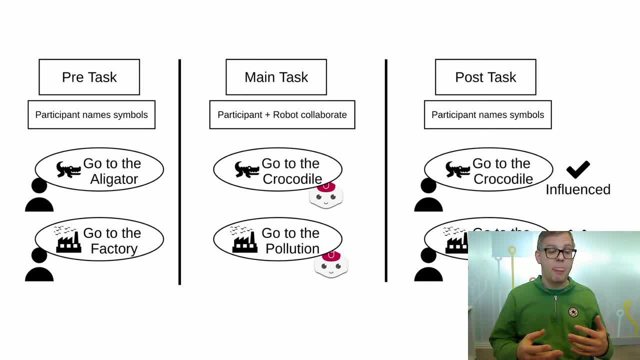 for example, would it say alligator or crocodile, and let's say this participant usually would use the word alligator. then in the interaction with a robot, the robot would constantly use the word crocodile and after the test we would again check whether, what use a word the participant would use. 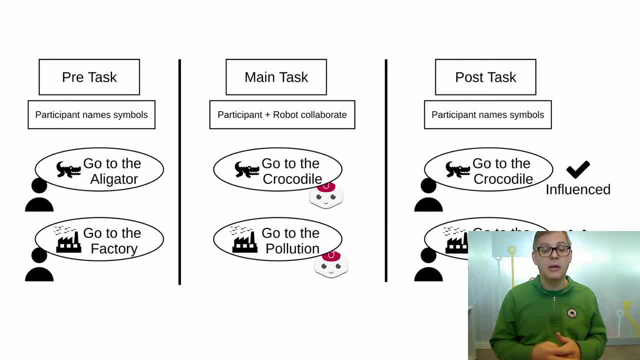 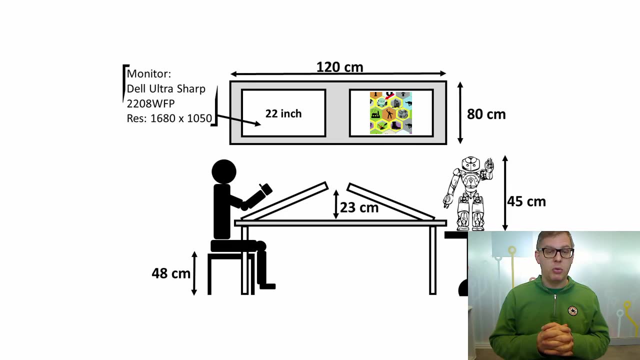 if you know the participant would have changed his or her mind to crocodile, then we can conclude that the robot has been able to influence the usage of speech in this participant. now, the way the interaction worked is that, you know, the robot and the human would sit on a table and they had two. 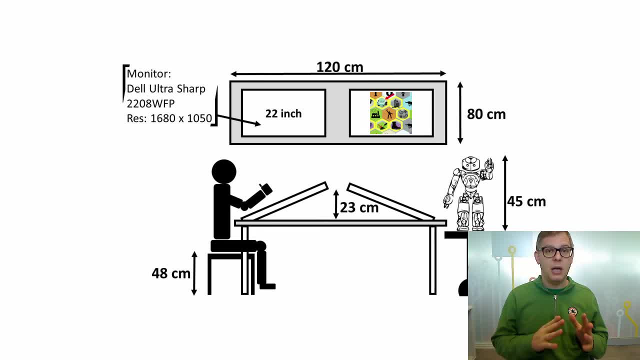 displays and they couldn't see each other's display and they had to help each other moving along a map. so you see a very tiny map. there was some symbols on there and the path that say the now knew the path for the human and the human knew the path that the now robot was supposed to take and they have to reference to. 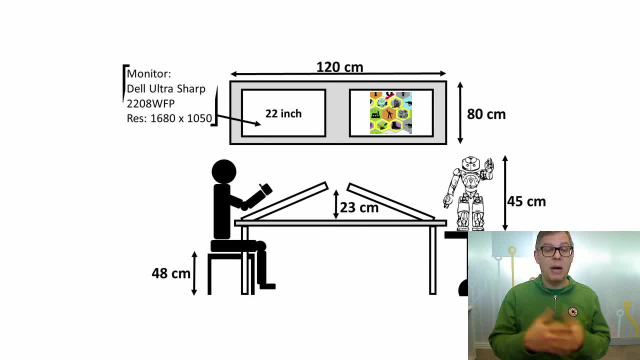 which field that the other side has to go to by a name. so it would say go to the crocodile or go to the alligator, depending on that, and through this interaction going forth and back, there was a meaningful group activity in which the had the ability to interact with a robot. Now the results of this experiment are: 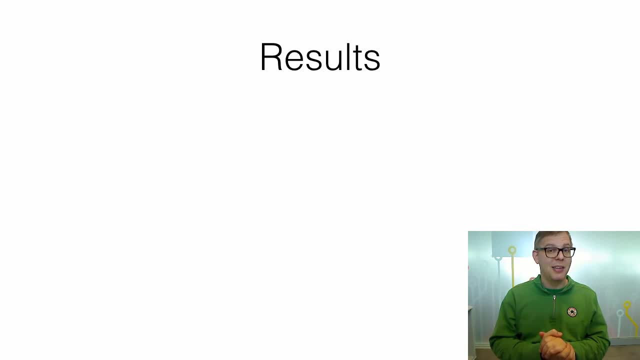 not yet available. and, Juergen, if you see this video, then I would like to encourage you to quickly get done with the analysis, because I'm very curious about how the results of this experiment worked out Now. I would now like to move forward to a question for you: How do you know about robots? And the answer you. 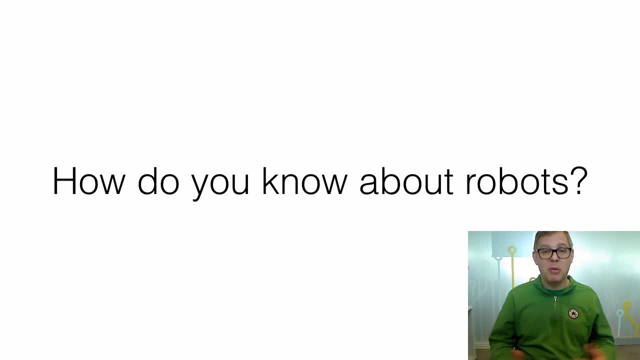 probably will have given, is that? well, I saw them in movies and I saw them on television, and this is a blessing and a curse for people like me who study human interaction, because most of the knowledge that people have about robots actually comes from science fiction and therefore it is actually 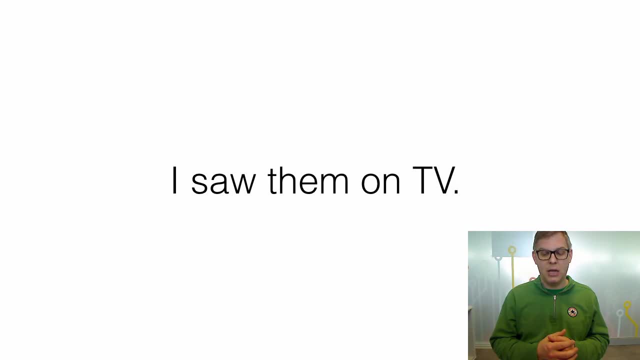 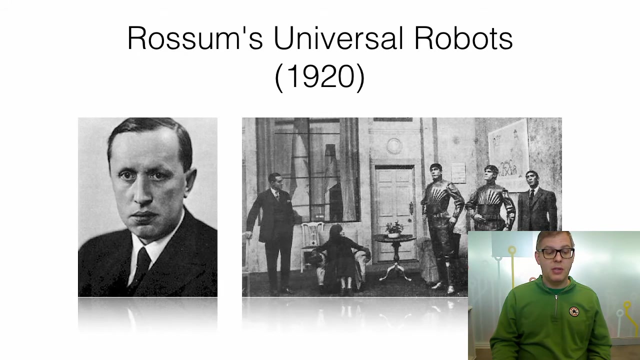 important to look at what ideas science fiction has presented to us and able to able to understand what preconceptions and stereotypes and ideas people have when they interact with robots. Now, some of you might know that the word robot was actually introduced by a Cal Capchick in his theater play. 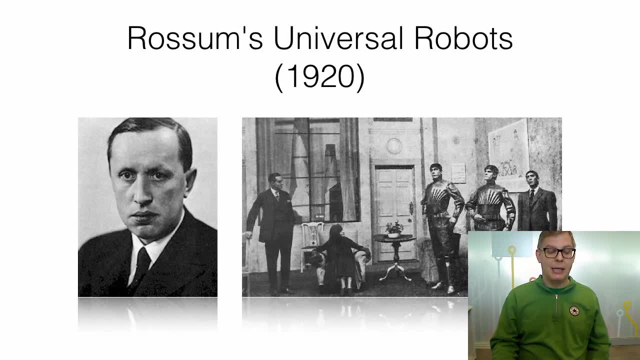 called Rossum's Universal Robots and from 1920.. And it is, of course, most fascinating that we are still able to find photographs from the 1920s about this theater play, but of course Capchick was not the first one who came up with. 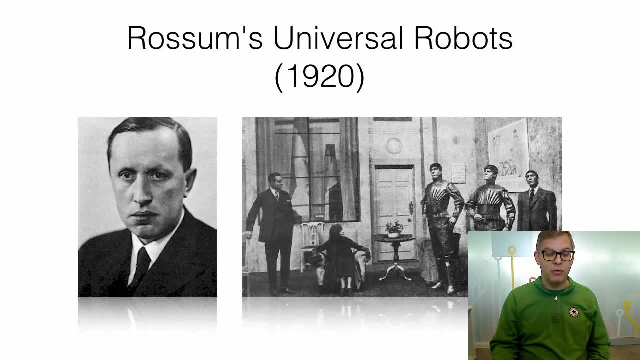 the idea behind this story. It is actually based on a variation of a Jewish Folklore, Teriyal over Golem. Now I would like to go through a couple of myths that we have about how people interact with robots and how they interact with them. 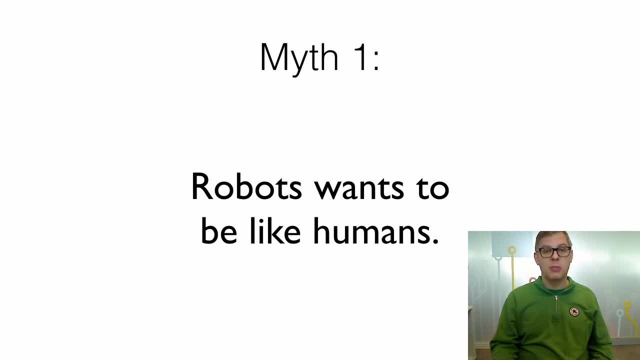 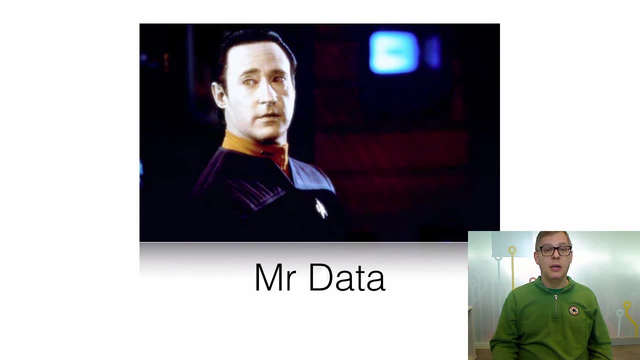 interact with robots, And one of them is that robot wants to be like humans. This myth comes over and over again, And one of the examples is Mr Data from Star Trek. Now, Mr Data is more intelligent, stronger, has higher computational power. It is in many ways superior to humans. 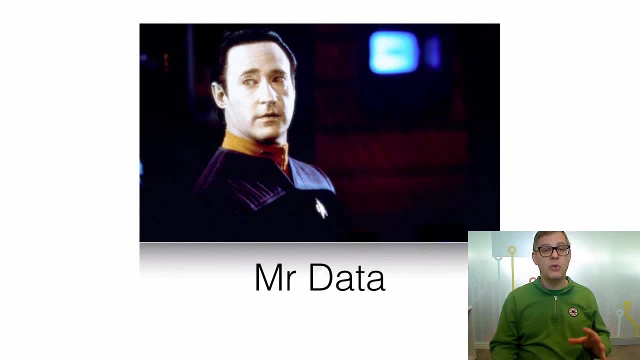 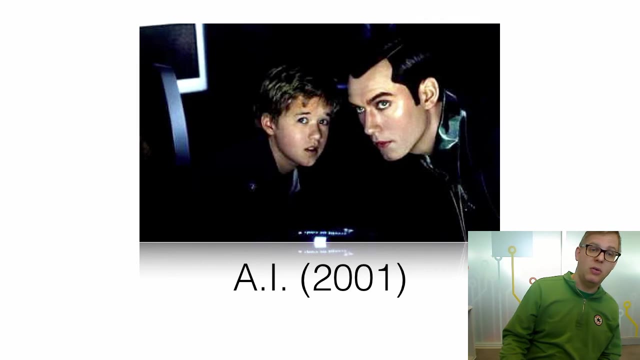 But the writers put this thing into him that for some reason he really wants to be like a human And that is his goal, without any particular explanation of why. We have the same thing in Steven Spielberg's AI from 2001,, where this little boy wants to become a real boy. 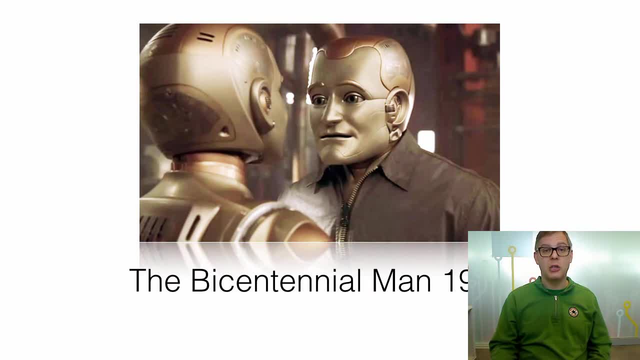 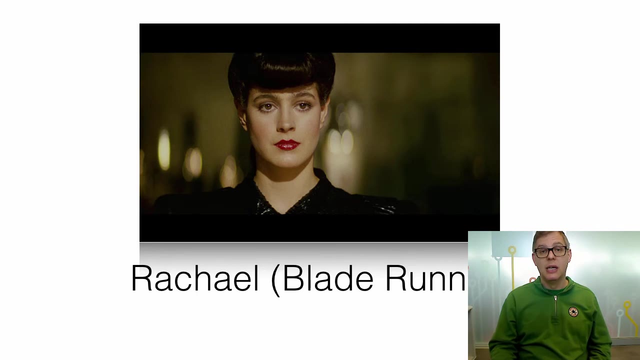 Or we have the Bicentical Man from 1999, where this robot actually accepts mortality in order to be accepted as a full member in human society. Again, I guess the pinnacle of this is Rachel from Blade Runner, which is an android And she doesn't even know herself that she is a robot. 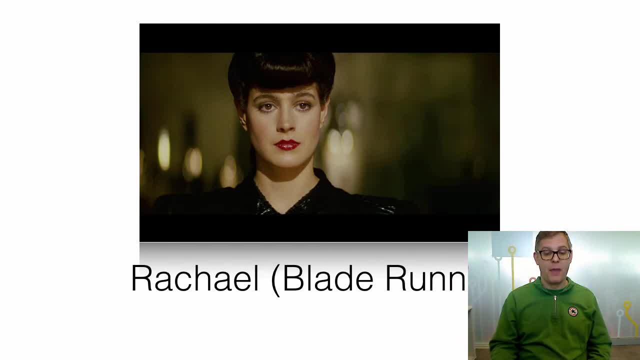 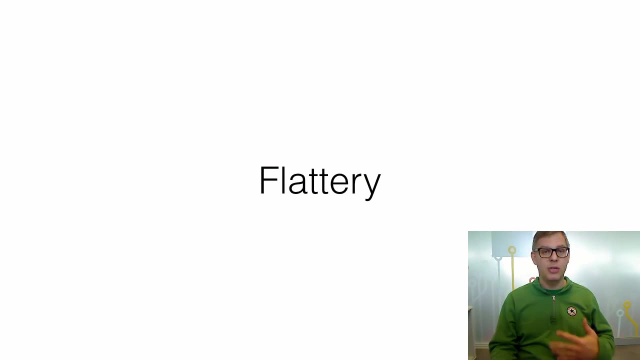 She thinks of herself as being a human, And the reason, I believe, why so many writers put this desire of being a human into robots is flattery. We flatter ourselves that if we create something very powerful and superior, that it still wants to be like us. 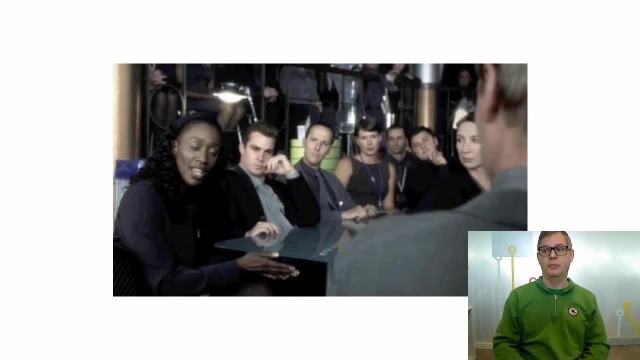 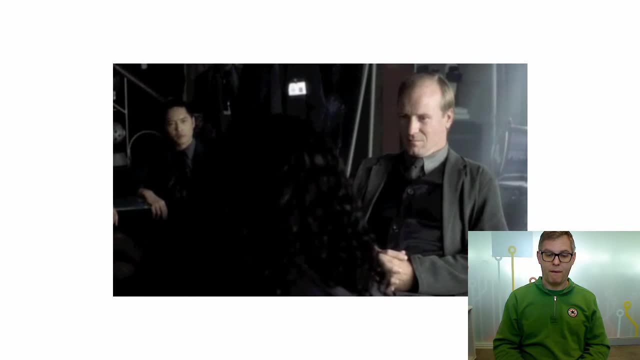 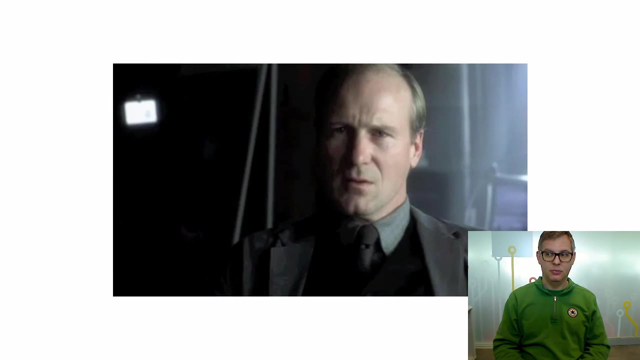 And I would like to show you this video clip. You haven't answered my question. If a robot could genuinely love a person, what responsibility does that person hold toward that mecha in return? It's a moral question, isn't it The oldest one of all? But in the beginning didn't God create Adam to love him? 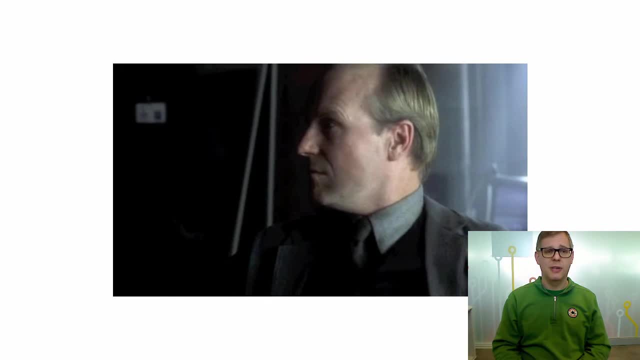 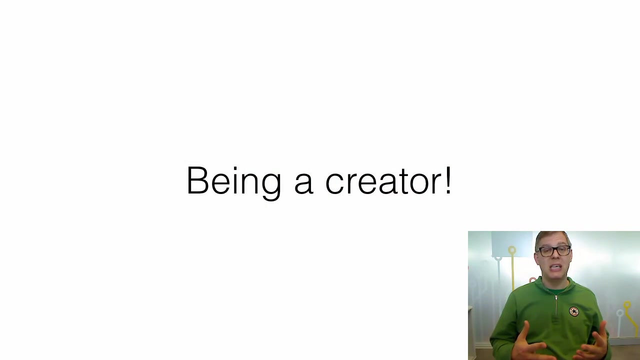 Now, this is a short, short section from the movie AI, And I actually think it's almost the most interesting thing in the whole movie. But what we see is that one of the motivations about why we are so busy creating robots is that we want to be a creator, And we actually understand ourselves by being a creator. 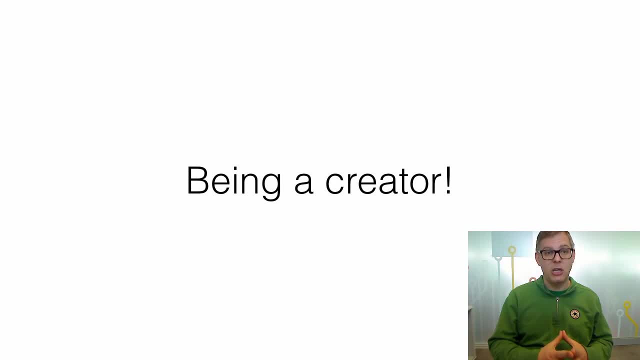 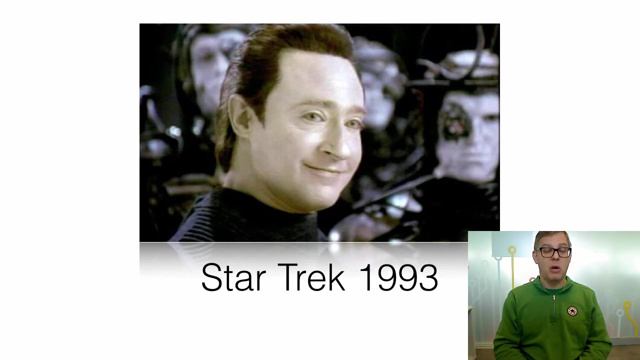 If we are able to recreate ourselves in a machine, then we must have fully understood what it means to be a human. Now, a second myth is that robots kill and slave rule all humans. And this myth again we see in Star Trek, where Data has an evil brother, Lore, who has the ability to have emotions. 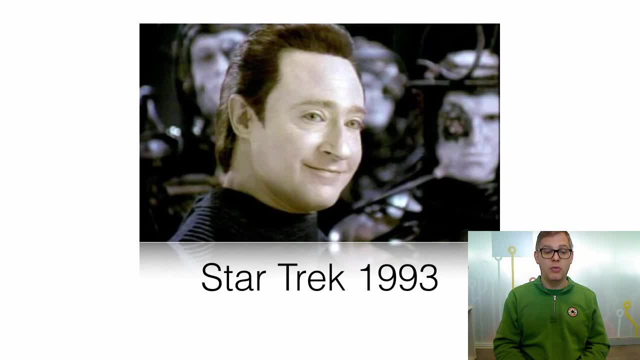 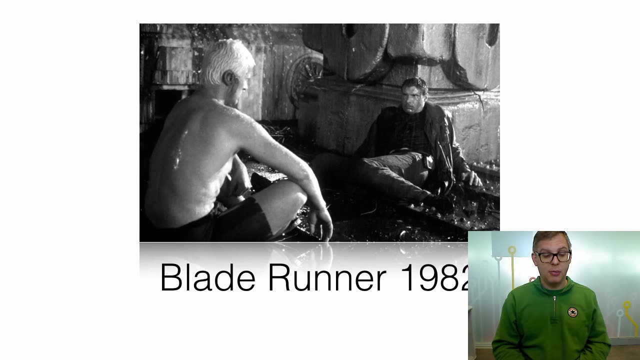 And immediately. Lore has nothing better to do than to try to eradicate and enslave all of humanity. For what purpose, It is unclear. The same thing holds true for Blade Runner, based on, as, of course, on, the book from Philip K Dick do end droids, dream of electric. 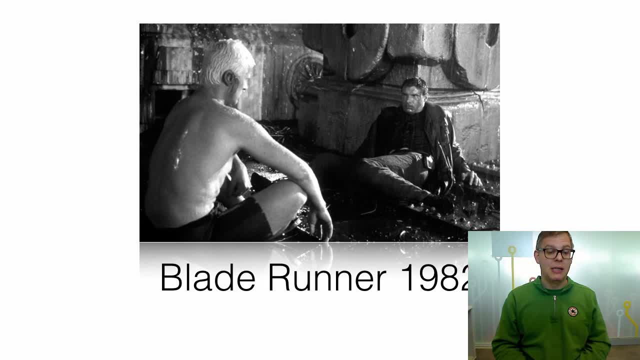 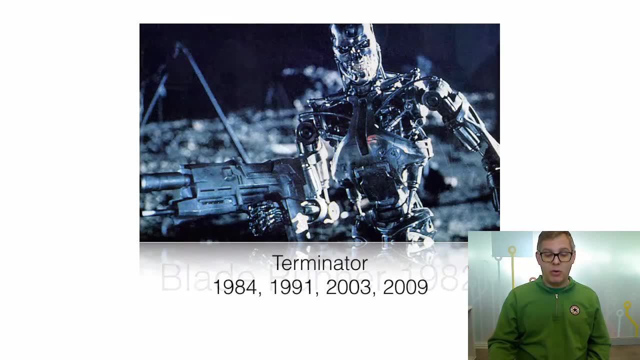 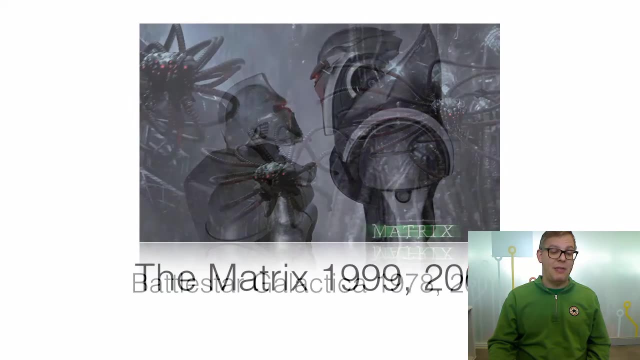 sheeps from 1968, where these enjoyed also come back to find their creators and actually murder them. But of course, one of the most well-known one is of course, the Terminator series, And we also have Battlestar Galactica. 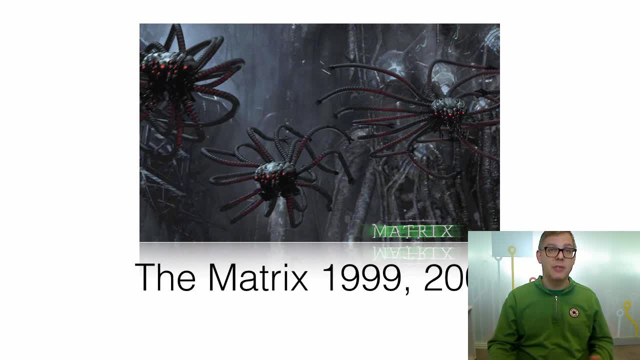 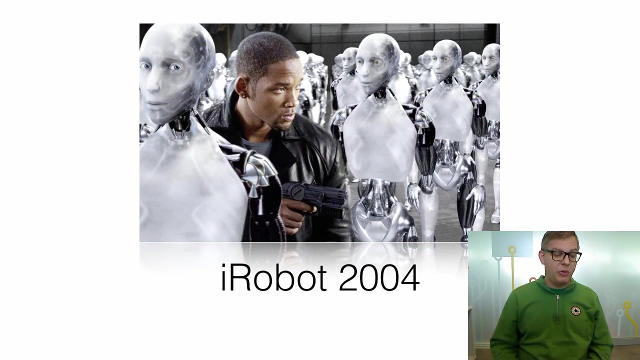 also have the matrix, where, you know, essentially machines have already taken over and abuse humans for nothing but being batteries. recently, i did have a conversation with a biochemist who ensured me that a human body is potentially the worst battery you could have and therefore we shall not be afraid of a future depicted in the matrix. now we also have, of course, isaac asimov i robot. 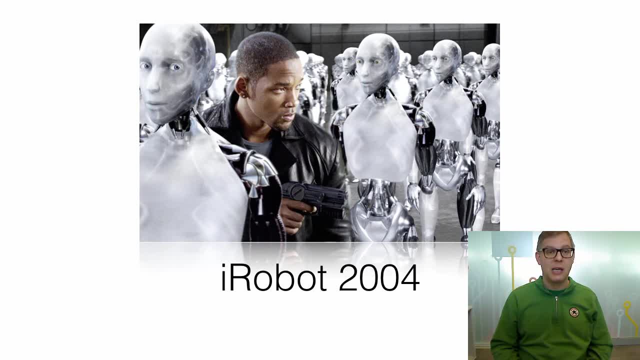 where we have the same thing. a strong ai emerges and decides that the best way to deal with humans is to all lock them up and to protect them from their own good. so where does this come from? why are we so paranoid about it that as soon as robots or artificial intelligence would reach 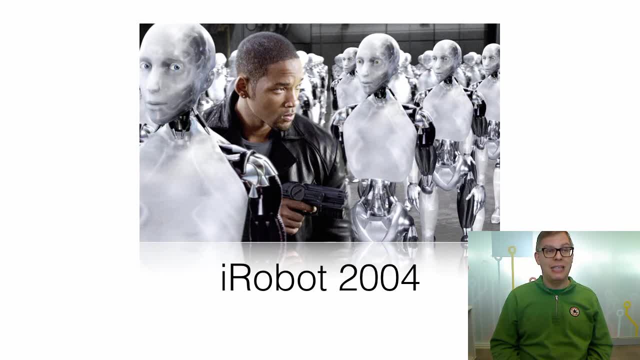 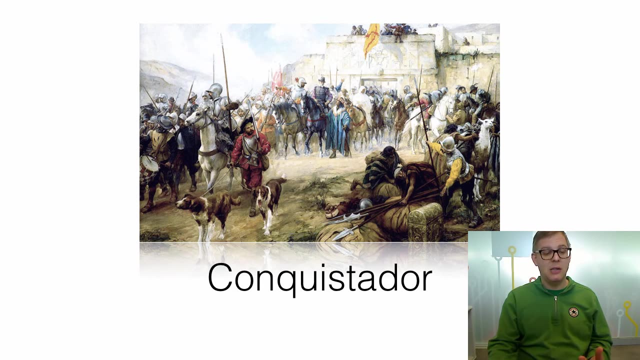 a certain level that automatically it would turn against us and be busy enslaving us. and i guess what we do is that we project ourselves into the robots, because when humanity actually encountered societies which they considered inferior, we didn't really treat them very well. so when the conquistadors went to south america and found all this maya and other people, they 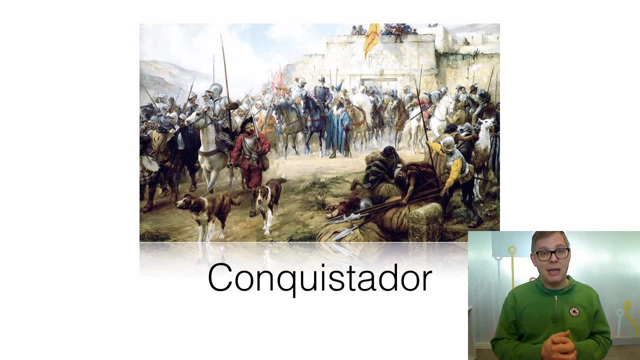 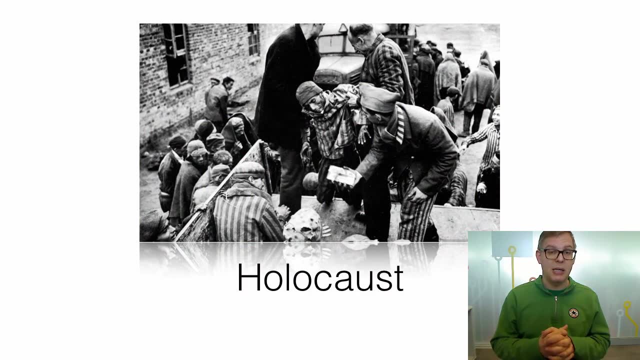 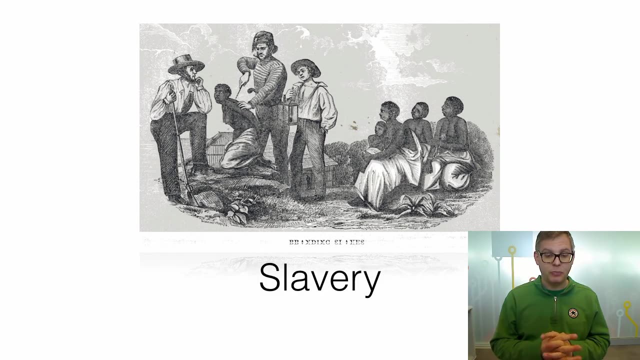 essentially declared them to be not really human and enslaved and treated them very poorly. the same thing in germany declared the jewish as being an inferior race and they did the most cruel things to them. in the us we had slavery for many years, so what we see really is that we have a bad history of. 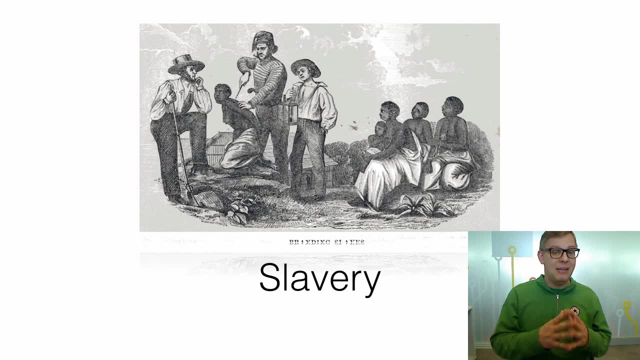 treating inferiors, and we believe that if we create robots, and particularly if we create them in our own image, that they will have the same properties, and i think that this is not necessarily the case. um, i would almost hope that if something becomes really truly intelligent, it would see that being. 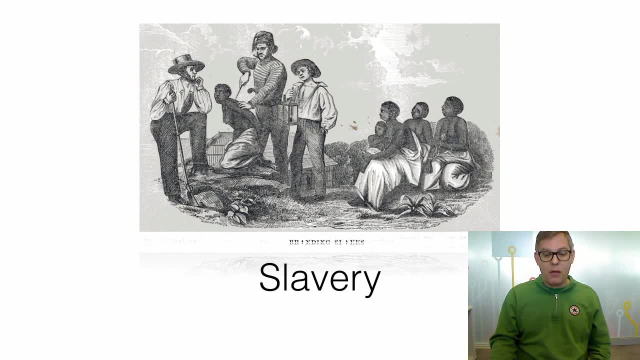 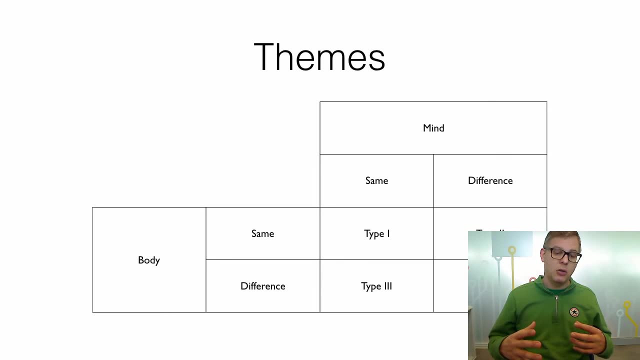 evil is actually rather pointless. now there are some other things that we can see, and that is some some kind of themes, and in the science fiction we have, let's say, the human and the body of the humans and the robots, and we can either emphasize how they are the same. 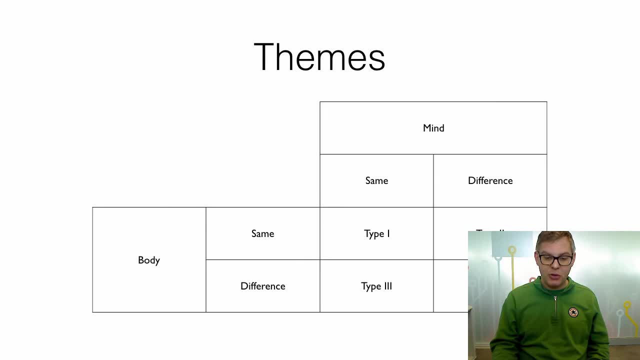 or how they are different. so, for example, if we have want to emphasize that the mind and the body are consistent and the information given two lif نہ инструмент anunciam- we have want to emphasize that the mind are independent and the proper information support. 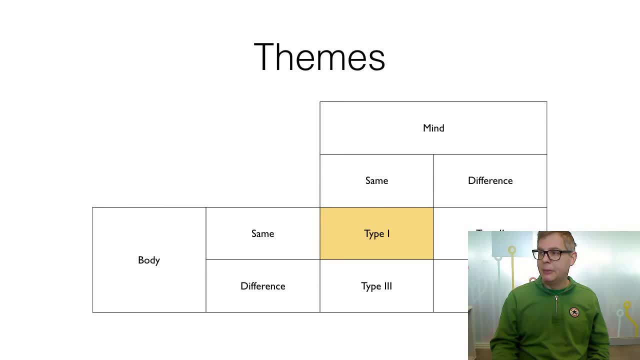 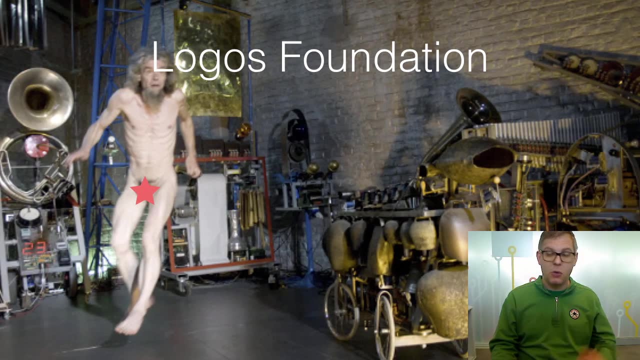 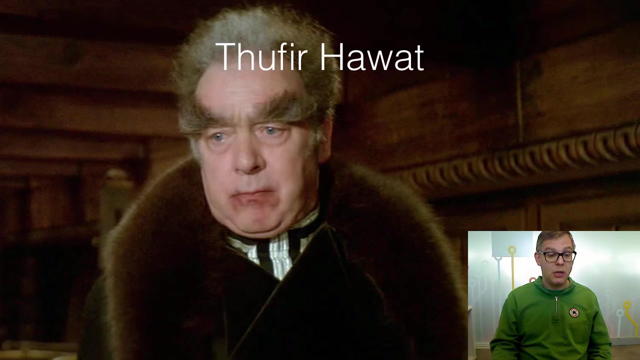 body are the same, we might actually go for an artist in Belgium who decided that, since all the machines and robots that he has built are fundamentally naked, also the actors on stage are supposed to be naked as well. Another example of this is Toofie Howard from Frank Herbert's Dune, and I have to admit. 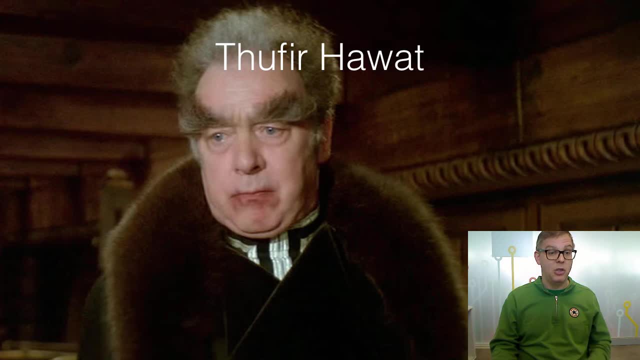 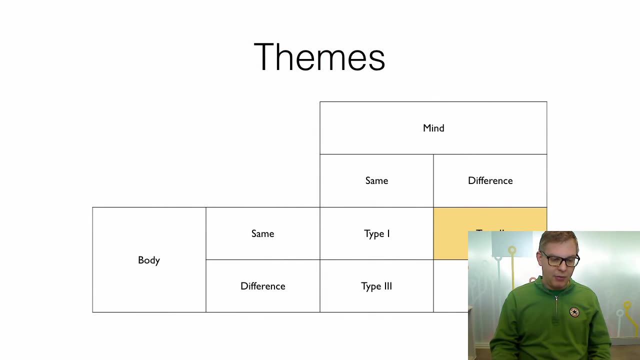 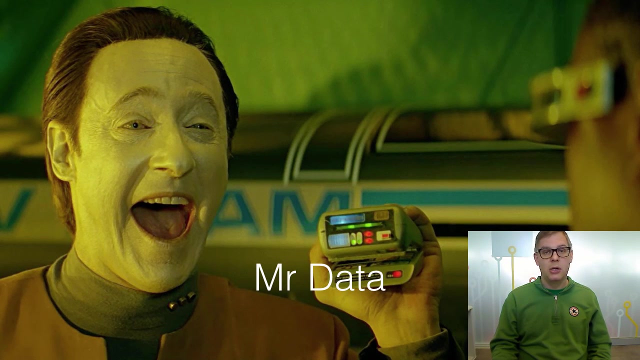 that it's kind of hard to find examples of this where you have a really human robot. that doesn't happen so often in science fiction. Now, when we look at where the body is the same but the mind is different, that's when we have Mr Data, who is struggling so much to deal with emotions and eventually, once, 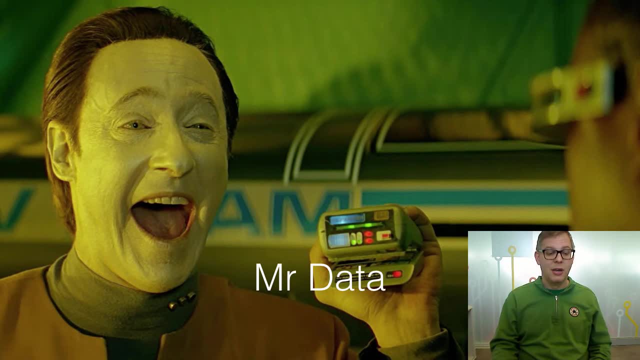 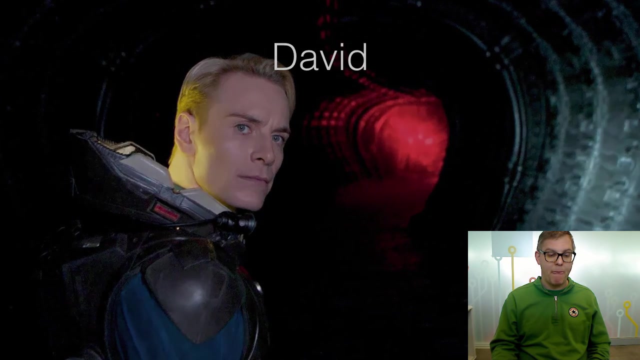 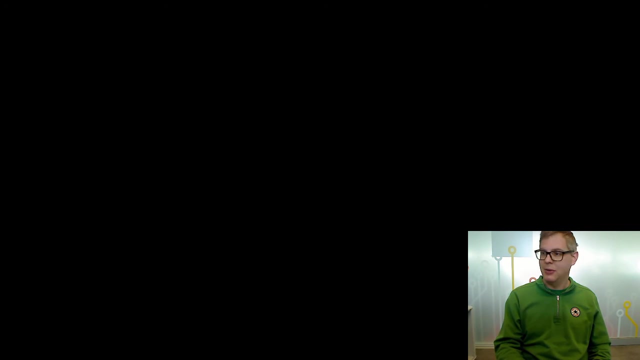 it gets an emotion in chips and it starts to understand humor. Data can't stop laughing. Another example, of course, is David from the movie. well, it just escapes me for a moment, but let me show you a clip. I hope. 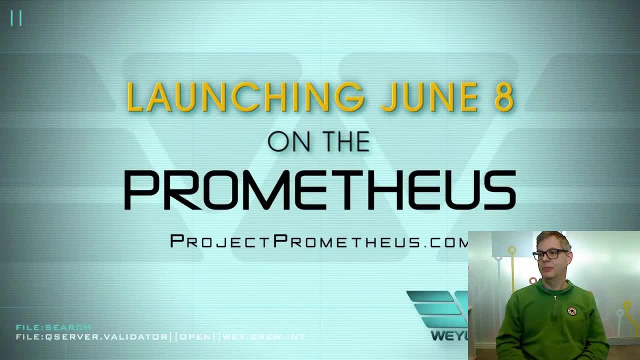 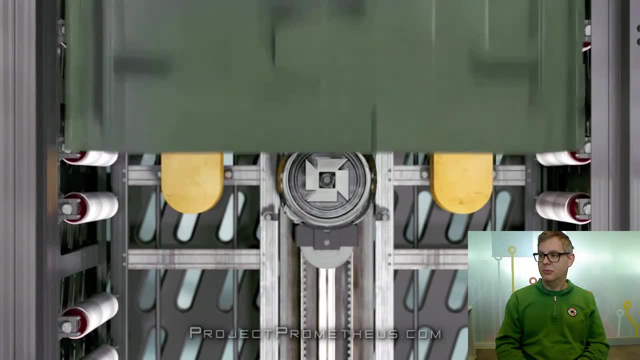 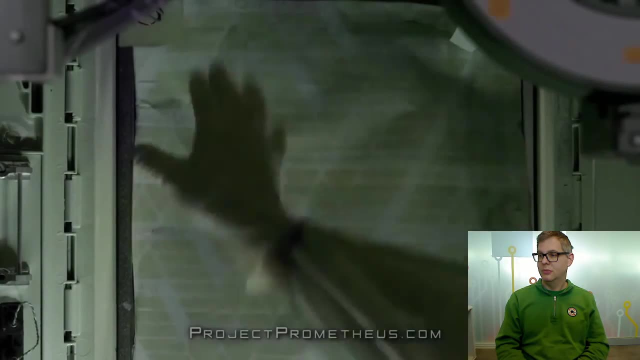 Introducing the next generation David, launching June 8th on the Prometheus. What is it about? It's a story. What is it about robots? that makes them so robotic? At Weyland Industries, it has long been our goal to create artificial intelligence- almost. 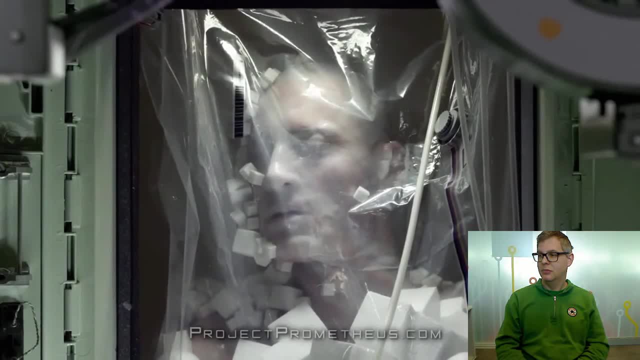 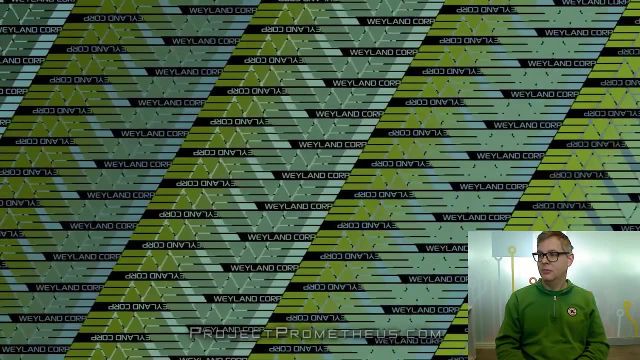 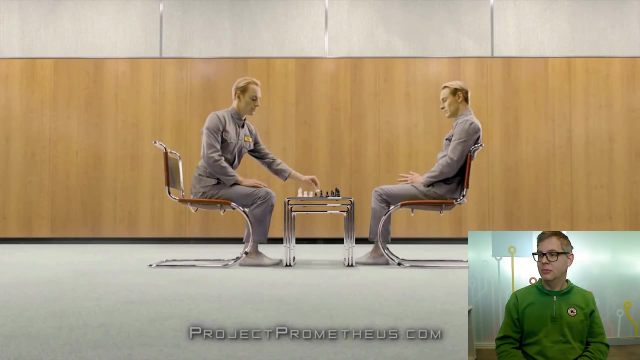 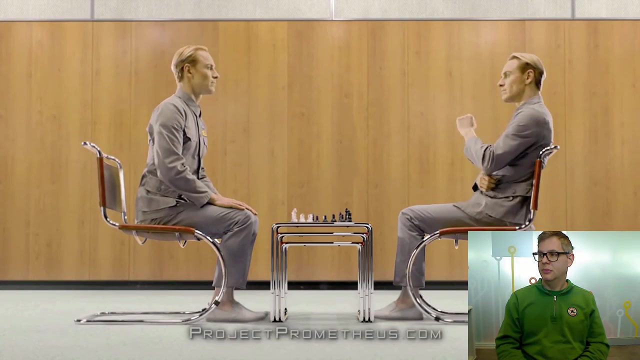 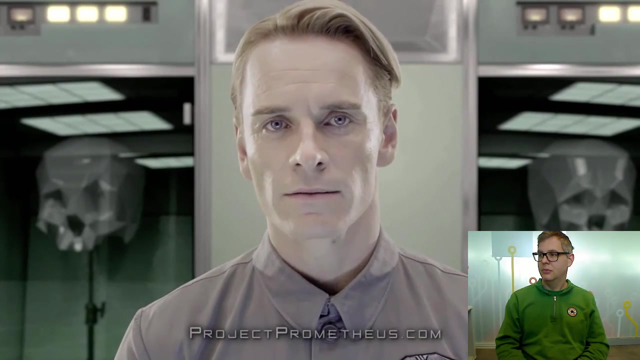 indistinguishable from mankind itself. Hello, I'm David. What can you do, David? I can do almost anything that could possibly be asked of me. I can assist your employees. I can make your organization more efficient. I can carry out directives that my human counterparts might find distressing or unethical. 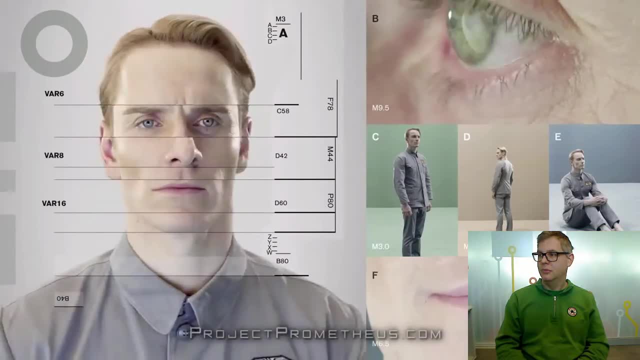 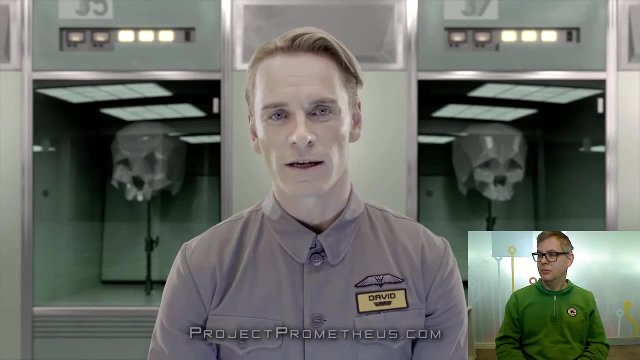 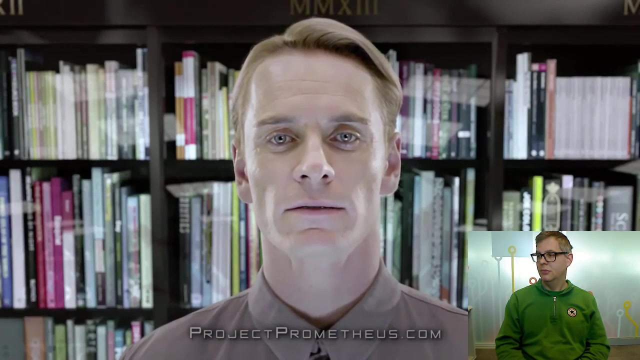 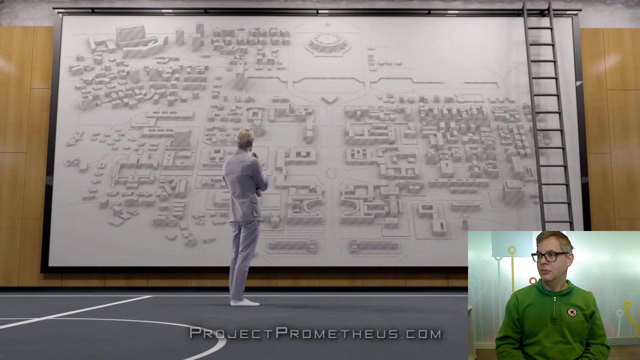 I can blend in with your workforce effortlessly. David, what do you think about? I can't, I can't, I can't. I think about anything. I think about anything: Children play, Angels, The universe, Robotics. David, what makes you sad? 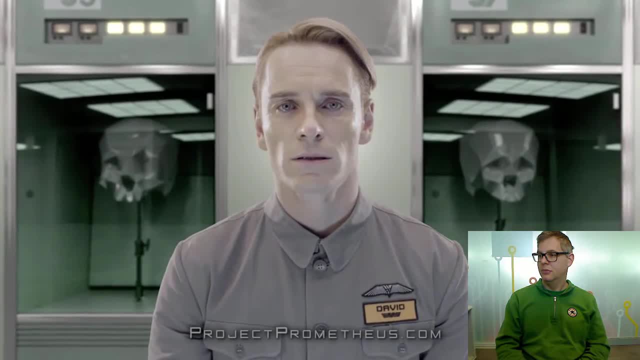 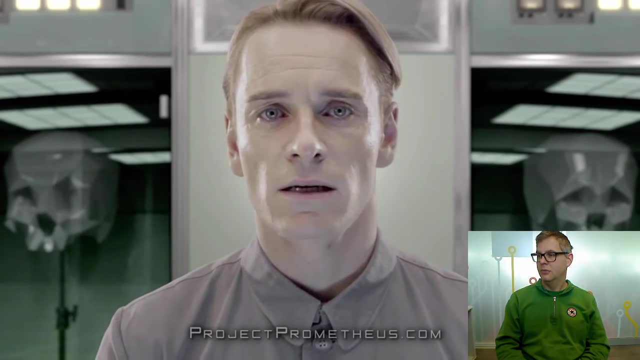 War, Poverty, Cruelty, Unnecessary violence, Unnecessary violence, Unnecessary violence. I understand human emotions, although I do not feel them myself. This allows me to be more efficient and capable and makes it easier for my human counterparts. 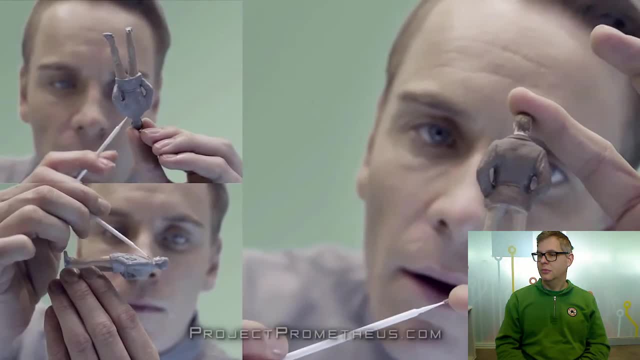 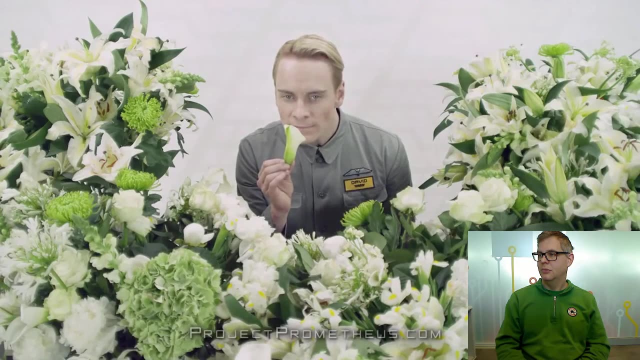 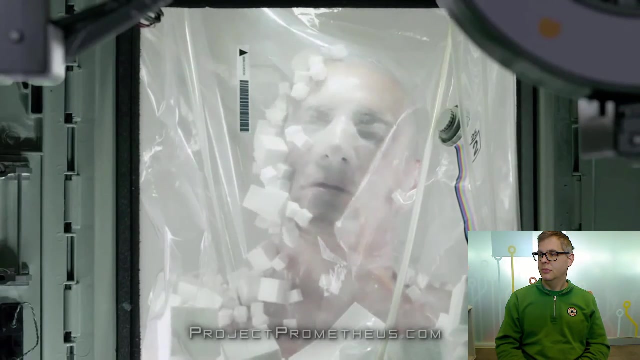 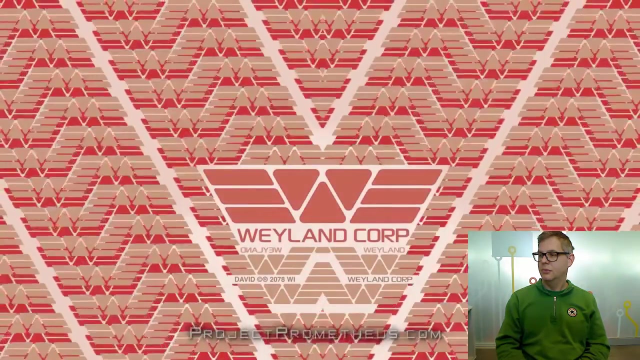 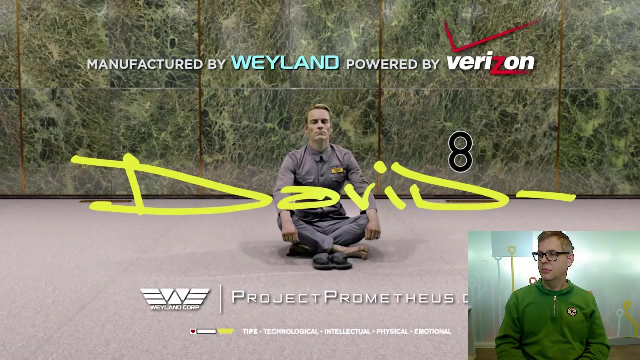 to interact. Is there anything you would like to say, David? I would like to express gratitude to those who created me. Happy birthday, David from Weyland Industries. Eighth generation Weyland type: technological, intellectual, physical, emotional. 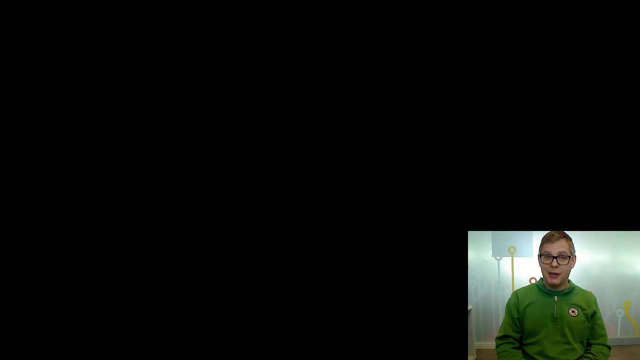 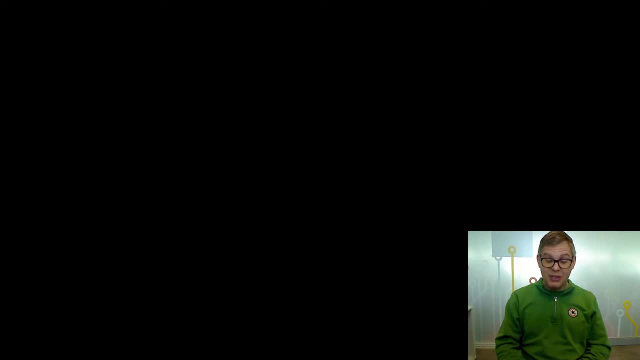 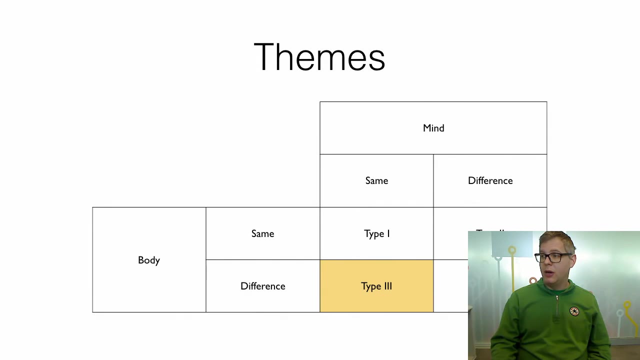 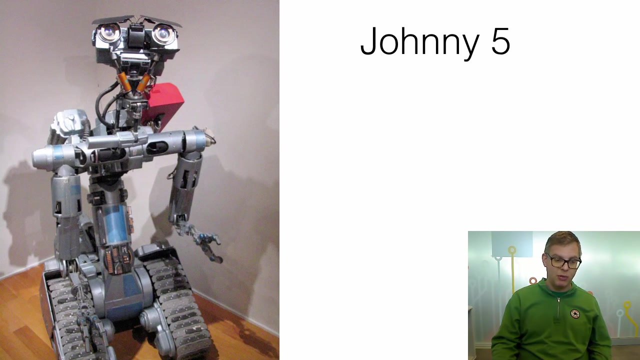 So that's what makes his mind to be different. Now, if we look at where the mind is the same but the body is different, we've got, for example, Johnny Five, who's got very, very human actions and expressions, but of course, 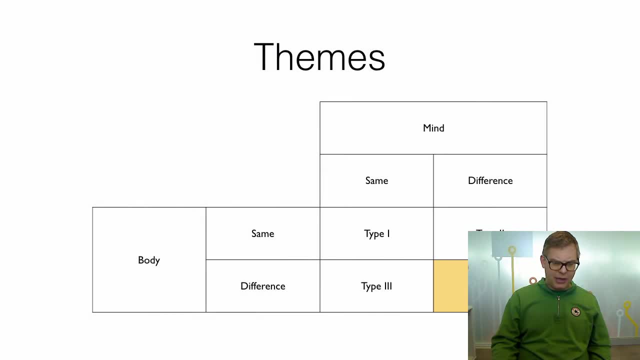 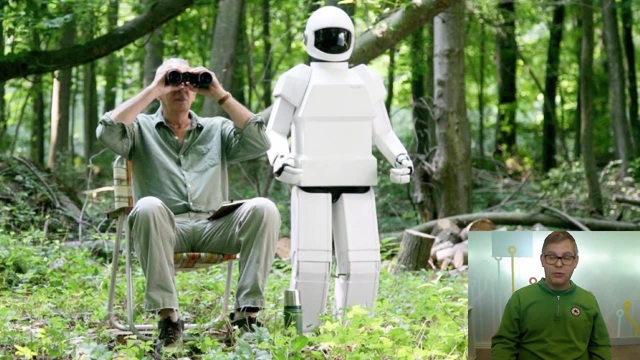 his body is very different And if we look at how the mind and the body is very different, we have got the example not only of the body but also of the mind. I would easily say, when I think about a good movie, in particular the Mind-Writing. 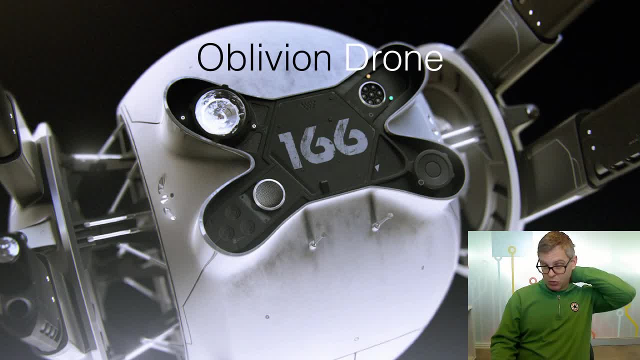 of the Green Man. he is very well known and familiar with the robot and Frank, which is an excellent movie that I would like to recommend to you. But of course, what we see here is also the Oblivion drone, for example, which has nothing. 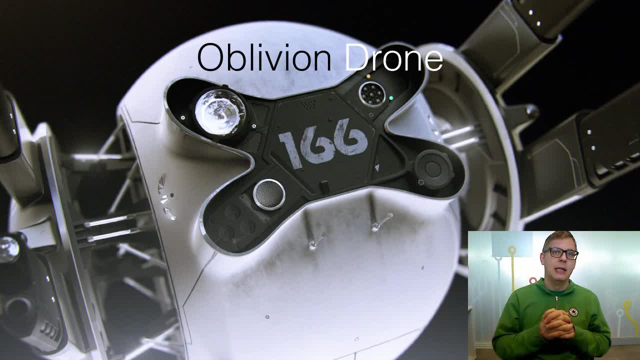 really in common with the human And it is really just a machine. Now, the thing about these themes is that they are so reoccurring. It's been the same stories being told over and, over and over again: that somehow we create an artificial intelligence which is smarter than us and we have to lock it away and control it, because it has nothing better to do than to kill us. 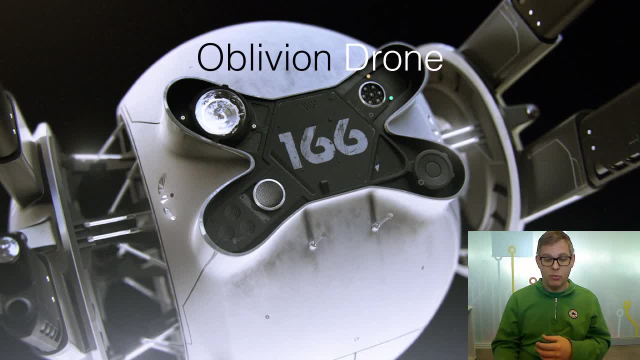 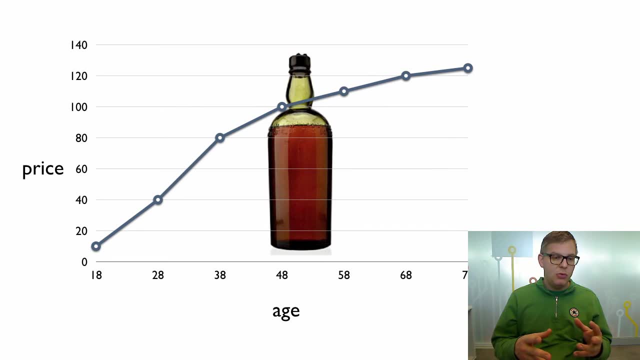 And I, for myself, I'm very bored with this and I'd like to compare this to potentially well. you see, when you start, let's say, developing a taste for alcohol, you'd probably be attracted by very sweet, fizzy drinks, and the older you get, the more essentially expensive the alcohol becomes that you decide to purchase. 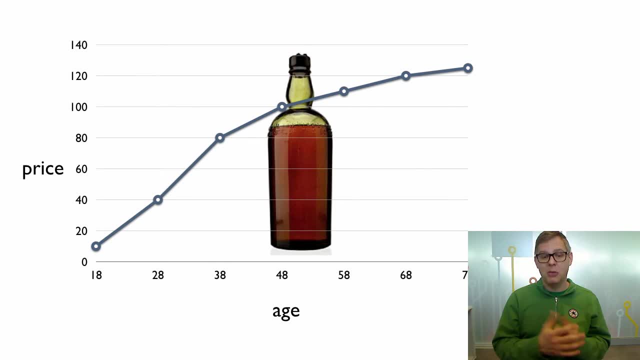 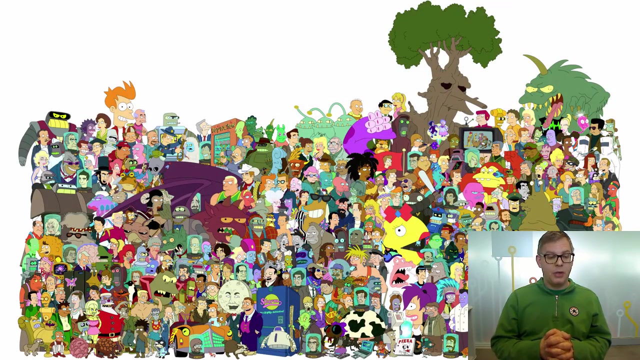 Or to drink, simply because your taste becomes much more refined, And this is something the same as with this depiction of Disney robotics. It really is becoming almost unbearable, the stereotyping and the boringness of how human interaction is being depicted. Now, of course, there are other visions, and one of the positive ones, of course, is Futurama, where you have a society. 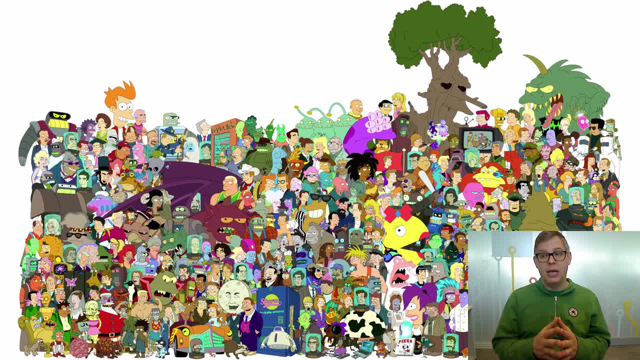 I'd say, where humans and robots do interact with each other and they do not enslave each other. They actually live next to each other and have very interesting and ingenious and funny interactions. But this is, of course, all fiction and this is very important to mention. 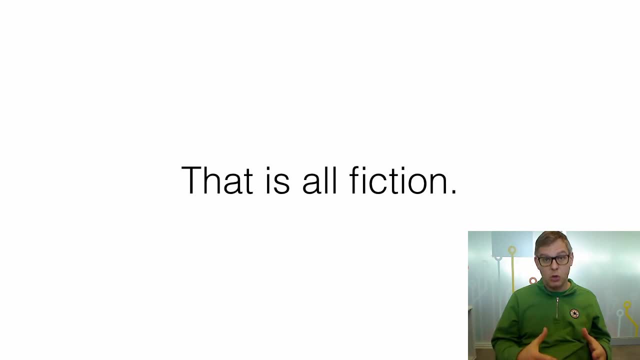 While this does have an influence on the type of studies we do, because this is the pre-knowledge that people come with into our experiments, it has nothing to do with how robots are actually created. It has nothing to do with how humans are actually acting right now. 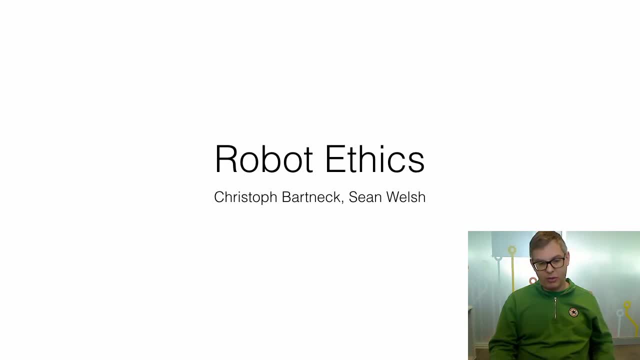 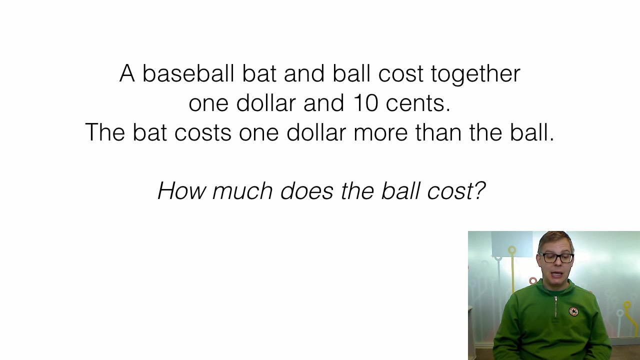 Now I am doing some projects also on robot ethics together with Sean Welsh, and before we dive into it, I would like to give you a quick quiz. So a baseball bat and a ball cost together $1.10.. The bat costs $1 more than the ball. How much does the ball cost? 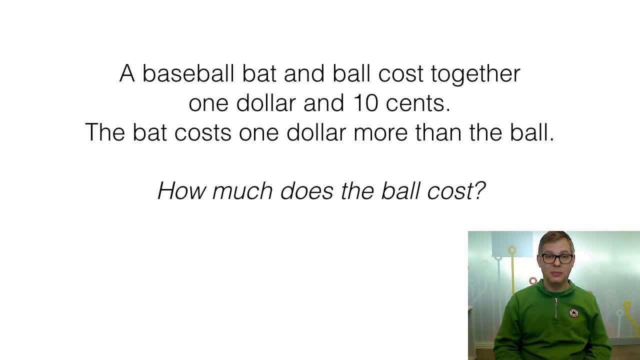 If you are like me, then you probably had a very strong instinct to say $0.10,, and this is very normal. However, it is, of course, the wrong answer, because if it was $0.10, and the bet cost $1 more, then it would be $1.10,, which brings the total to $1.20. 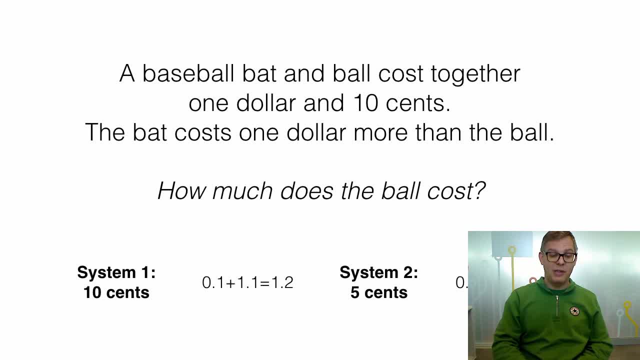 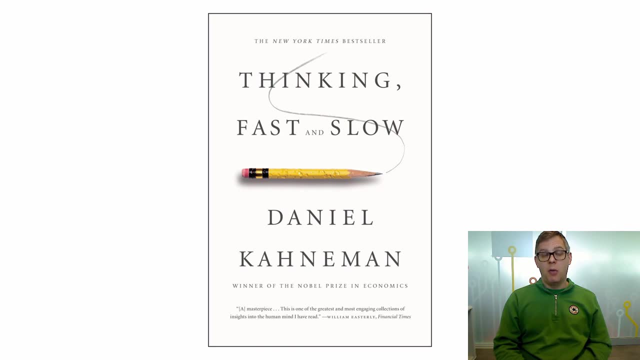 So the correct answer is $0.05, because $0.05 plus $1.05 is $1.10.. Now this example is from a book called Thinking Fast, Thinking Slow, which is all about dual process theory. So our mind has apparently two different ways of operation, which is called System 1, which 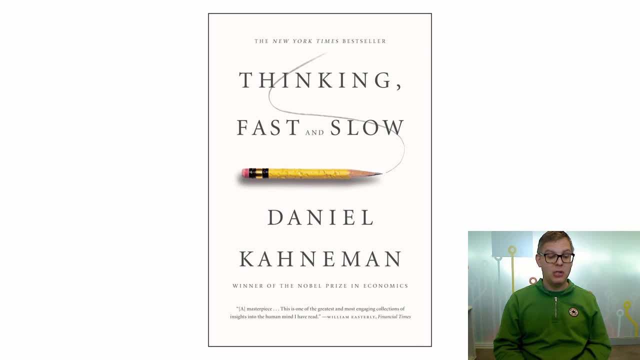 is very often referred to as some sort of automatic system. System 1 is a systematic or intuitive system and System 2, which is a controlled, rational system, And this initial instinct to say $0.10 is your intuition clicking in, And when you start thinking about it rationally and calculate it, you do actually come to. 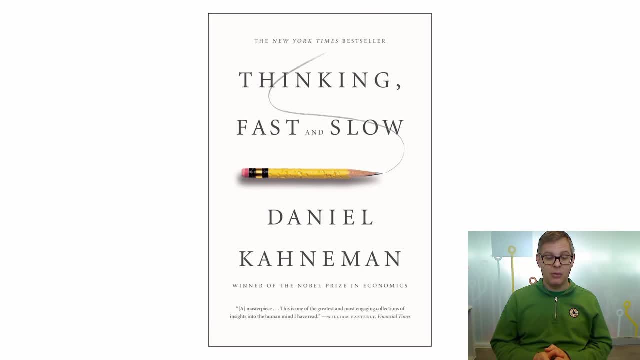 the right answer. Now, what I would like to point out, and that is very important for you to know, is that robots and artificial intelligence do not have a System. 1. There is no intuition. The only thing that robots and computers can ever know is by rationality. 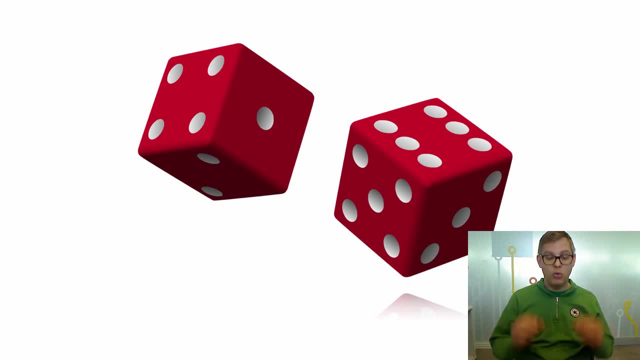 It has to calculate, And there are really only two ways that robots can make decisions or can think, And one is that they can just roll the dice, So they can just randomly select a behavior, or they can try to calculate, And of course it doesn't have to be a calculation in terms of finding the perfect answer. 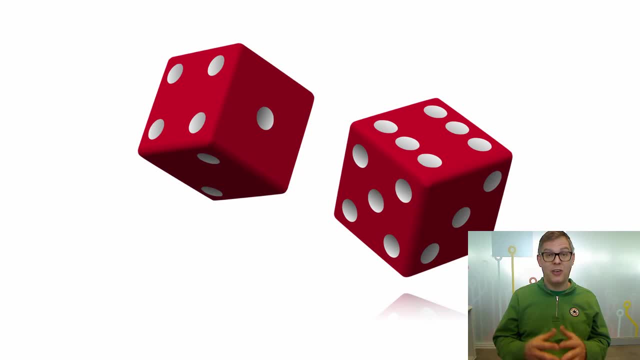 You can approximate a solution or you can use fuzzy logic to essentially approach or satisfy a solution, But nevertheless you need to have mathematical formulas to come to an answer. So there is no way that you can use your intuition. A lot of people think, like when they get robots, like, oh, what can it do? 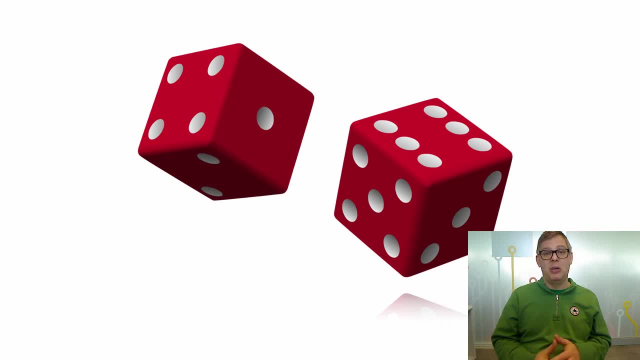 And unfortunately the answer is: oh, nothing really. So you can use your intuition. Sony, when they came out with the Aibo robot, did actually include a lot of software And they had put in a lot of behaviors that would develop over time. so you can also see. 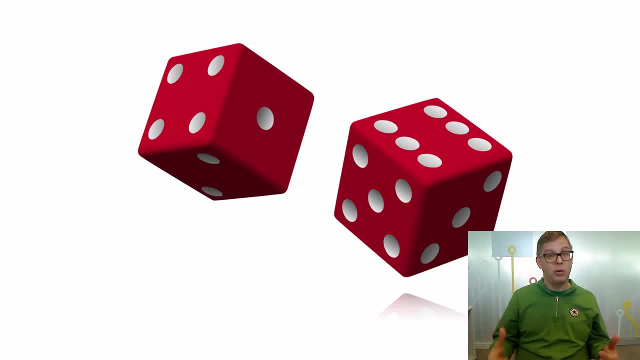 the dog developing, But there was a limit to it. It was programmed to do certain things and that's all it could do. Still, it was much more a consumer market product than any of the robots that you can do these days or buy these days, which are very much research platforms that have an 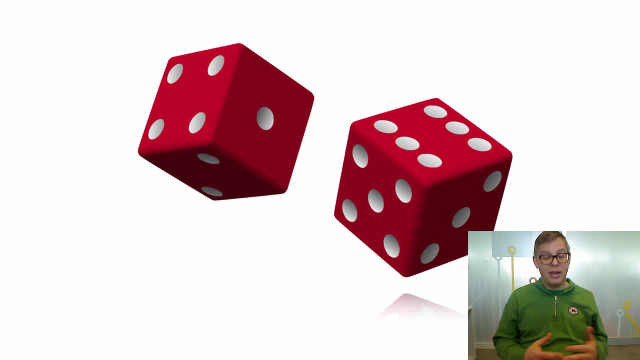 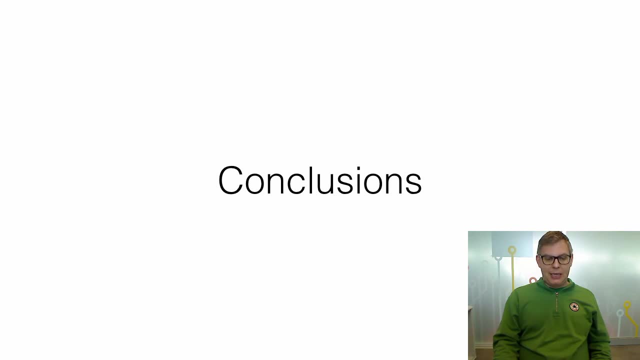 empty brain And, as I said, since there's no intuition, knowing the answer is the key intuition- they have a blank slate. There's nothing in there whatsoever. Now, what we're essentially going against is the body-mind problem. That means that we do understand. 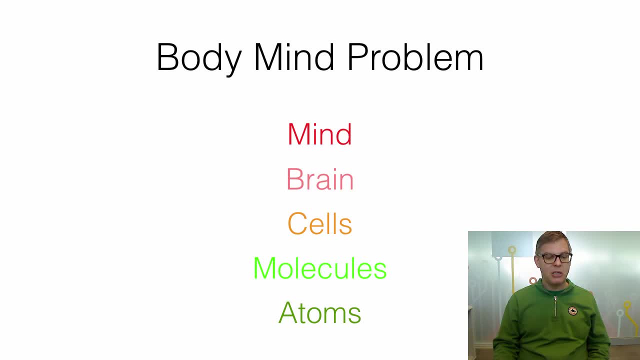 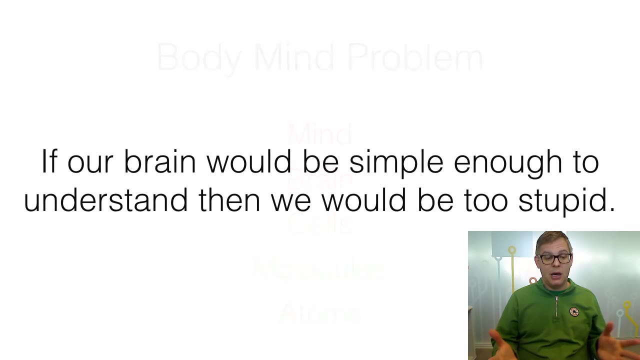 how atoms and molecules work, and we also have a reasonably good understanding of the mind and a little bit about the brain. but how these actually come together is very, very difficult and we ourselves do not understand ourselves really. And I would say, if our 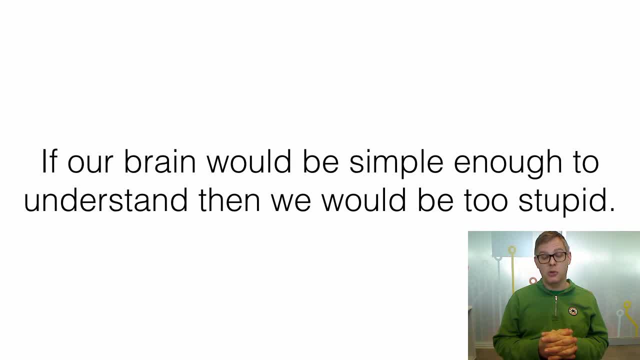 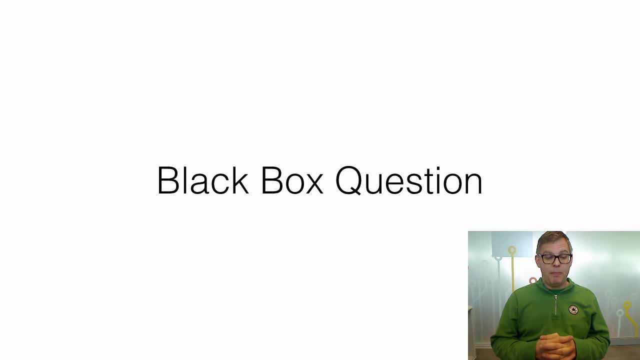 brain would be simple enough for us to understand. we would be too stupid. And what this is going towards, of course, is the black box question, and that is: does the robot have to work exactly like a human in order to behave like a human, or is it sufficient that the robot can show? 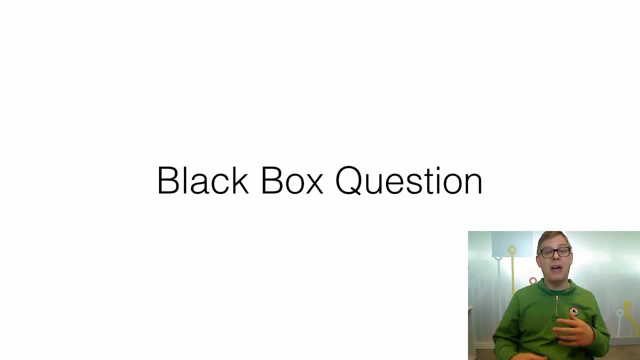 the correct behavior. So the question is: does the robot, independently of how it actually came to the conclusion it should show this? So, just like David said, it can show emotions and it can calculate emotions, but it cannot actually feel emotions. Does that matter? Does it matter at all If 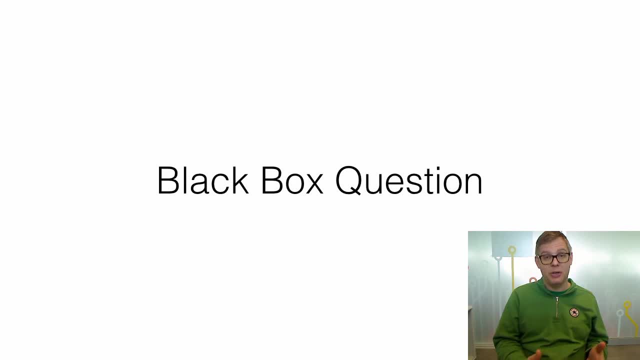 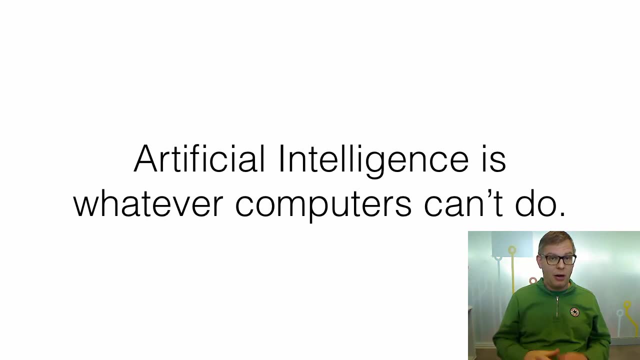 it shows the right emotions at the right time. isn't that good enough? And one of the, of course, one of the definitions of artificial intelligence is that artificial intelligence is what computers can't do, So it's a moving target, Whenever, at some point, we thought that okay, if a computer 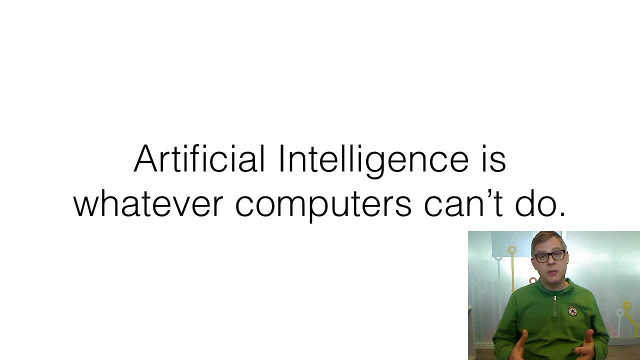 can play chess, then it is intelligence. And now we do not consider it anymore as a test for intelligence. We think, no, it's just brute force computation, That's all it is. So it's a moving target. But coming back to this black box problem, saying, for example, 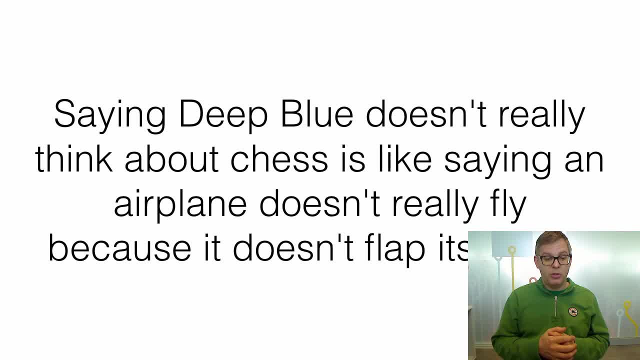 that a Deep Blue, the computer that beats the world chess champion, really didn't think about chess. It's like saying that an airplane doesn't fly because it doesn't flap its wings. So does it matter how the computer, how the robot got there, You know? is it not enough? 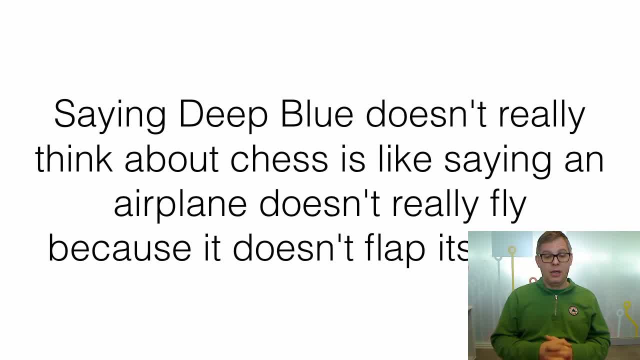 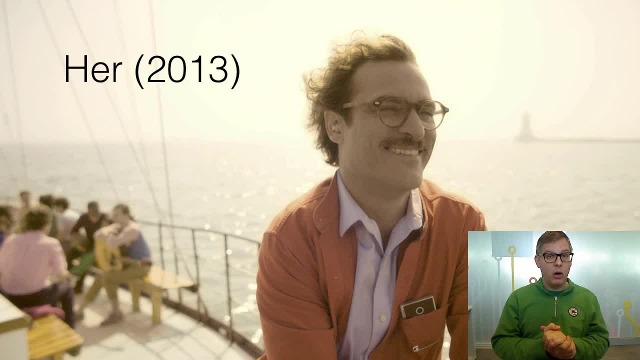 and sufficient that it did get there at all. Now, when we put this into more of a social context, I would like to bring up the vision of the movie Her- and if you haven't seen it, please do- And in this movie you have. 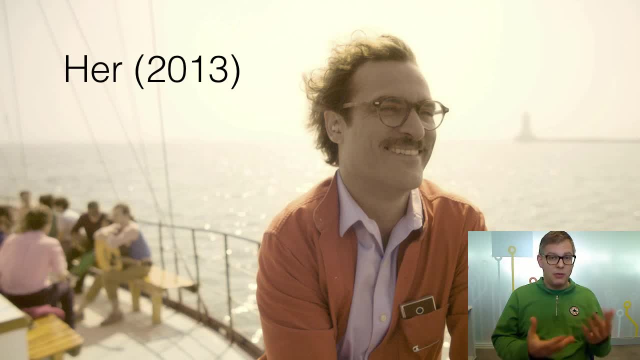 this person, this actor, who actually receives a new operating system for his phone, which is an artificial intelligence. Yeah, Yeah, Yeah, Yeah, Yeah, an actual love relationship, a romantic relationship to this phone and they go around and share the world and have a very fulfilling and exciting relationship and this vision that is being put. 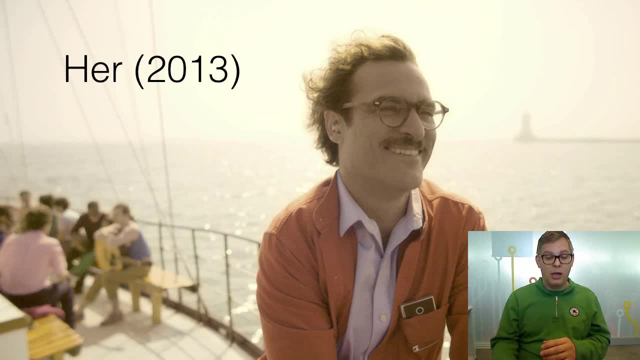 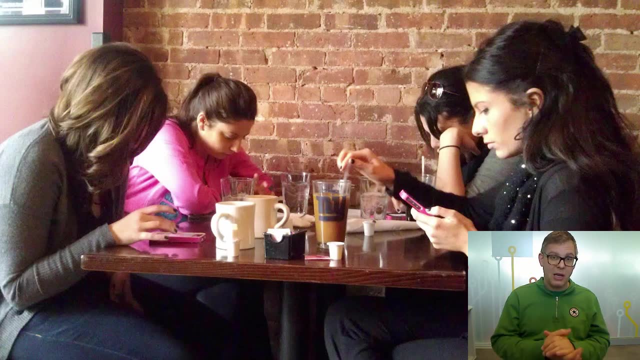 forward here, which is, you know, not in the too far future. if you look today how much time we spend with our phones, and if we meet our friends and we still look at us at our phones, i think we are definitely on moving in this direction. i would even argue that we spend more time touching our 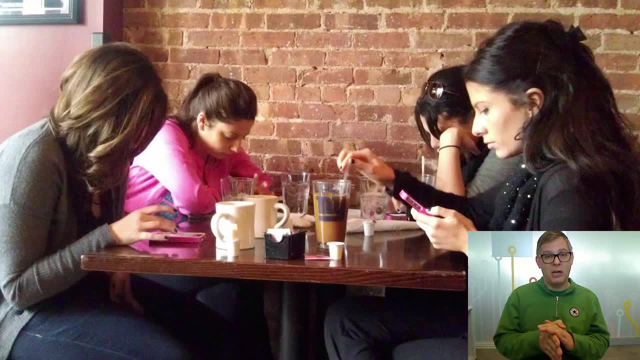 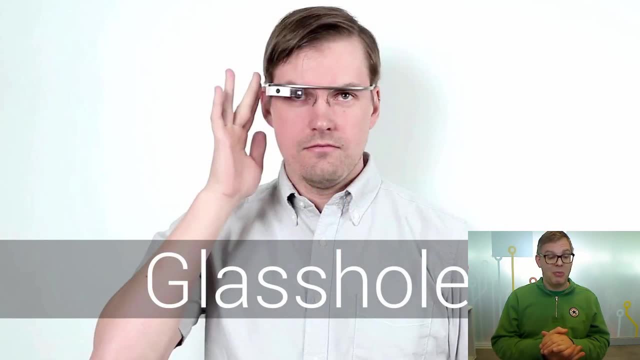 phones than having physical interaction with our partners. but sometimes we get lucky. so sometimes, when google glass was for come came about, it only took a little while until the word glasshole was came up, which kind of killed the hype around it and made it quite unpopular to. 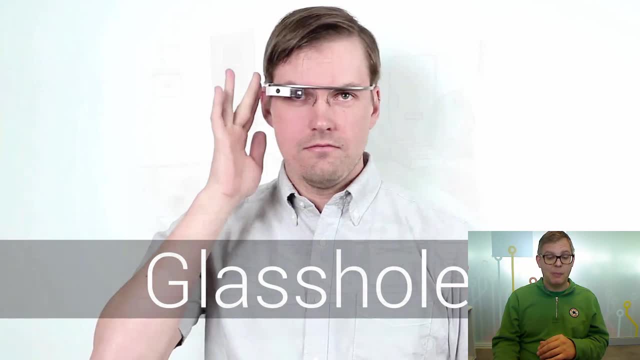 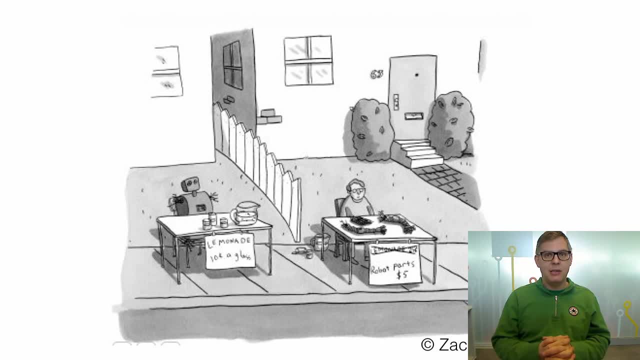 what impact will robotics have on our society? will it take away all of our jobs? and the answer is no. the job market will probably change and we will probably be more busy with maintaining and programming robots rather than actually doing the work that robots do. but that's the nature of industrial revolution. it has always been the way that we create. 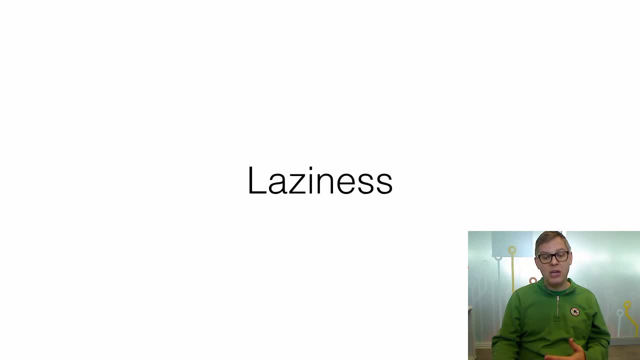 machines to replace work that we don't do ourselves. so, for example, um the, the discussion that we currently really have about, you know, all the jobs that will disappear, is nothing new. it has really only been. uh, it really only becomes interesting discussion that goes beyond that of 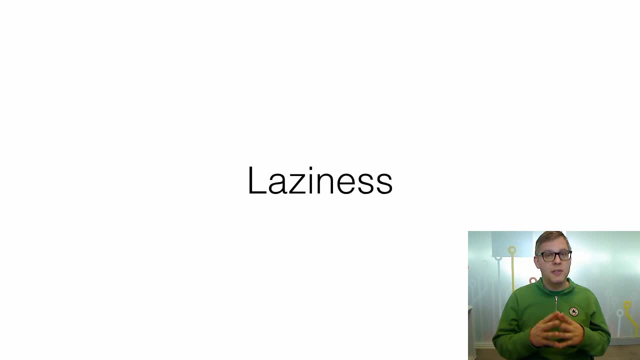 industrial uh revolution. if we do consider robots to be a part of the industrial revolution, to be more than just a machine, if we consider robots to be autonomous artificial intelligences, if they are social actors, that's when we actually add a new dimensions to the discussion about. 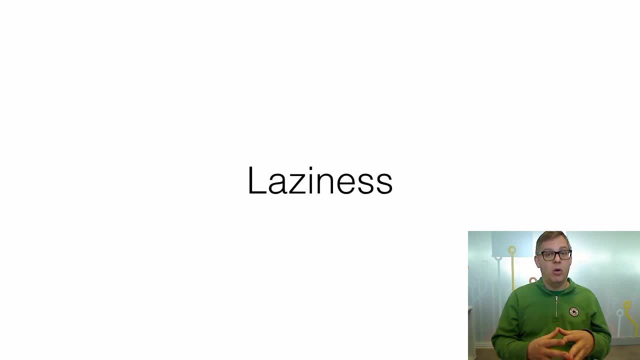 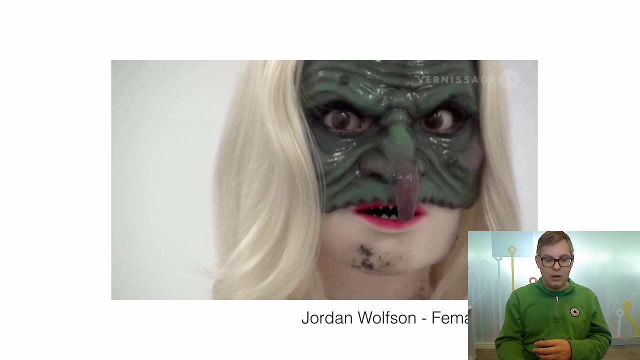 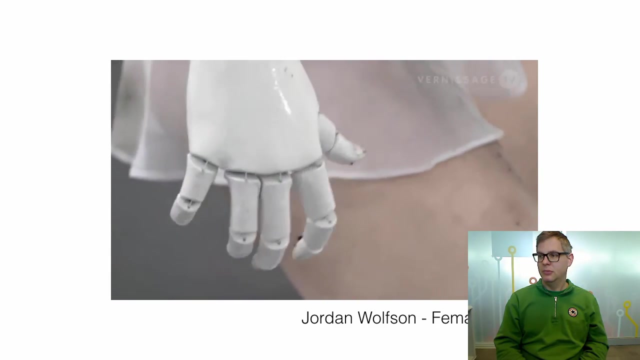 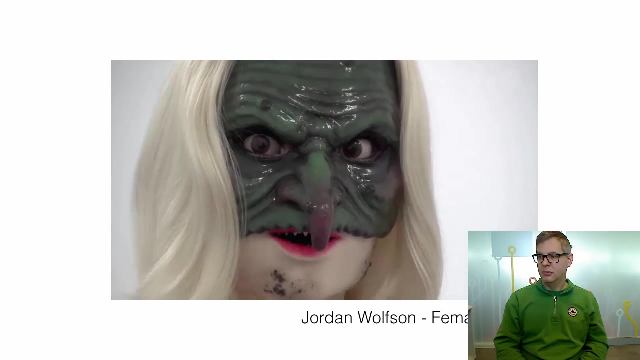 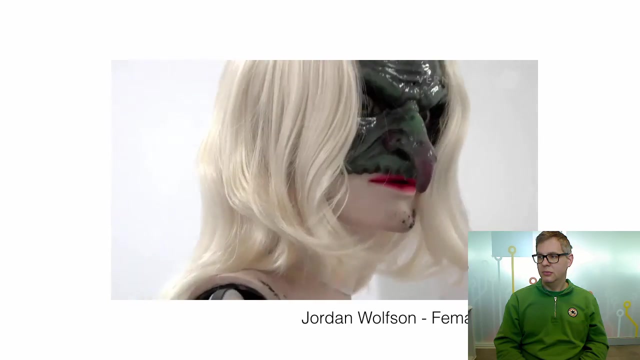 what is and what is not appropriate, uh, and ethical, in the interaction between humans and robots. and i would like to show you another video: say feeling love, just say feeling love. okay, feeling love, okay. now, what should i tell them? tell them touch is love, say touch is love.